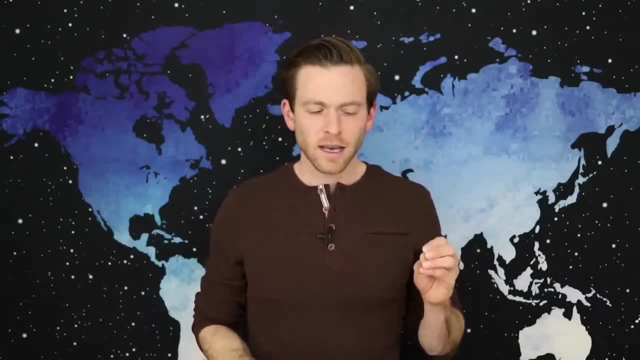 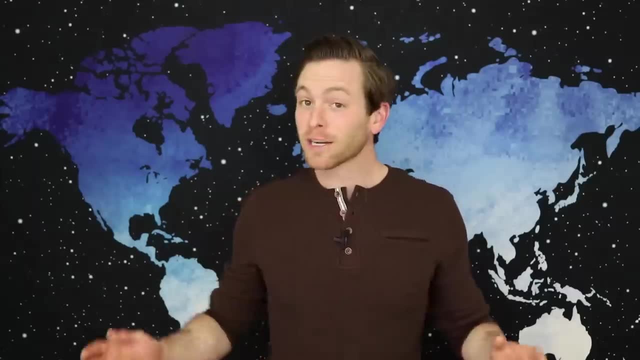 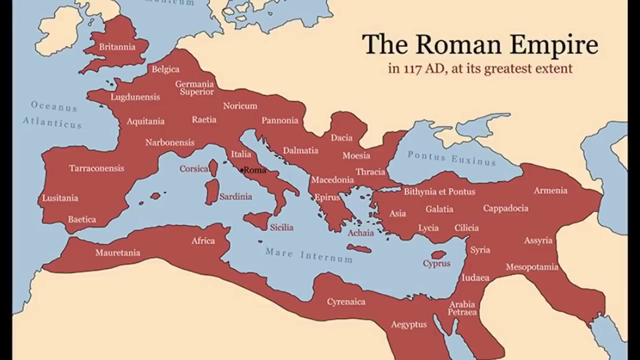 The widespread global extent of these similarities are what made my jaw drop, And I'm willing to bet that you'll never see these ancient sites the same way Ever again. Now, before I smother you with a couple hundred photos and comparisons, let me first preface this video by pointing out that the Roman Empire is considered to have been the largest and most widespread ancient civilization ever known to have existed. 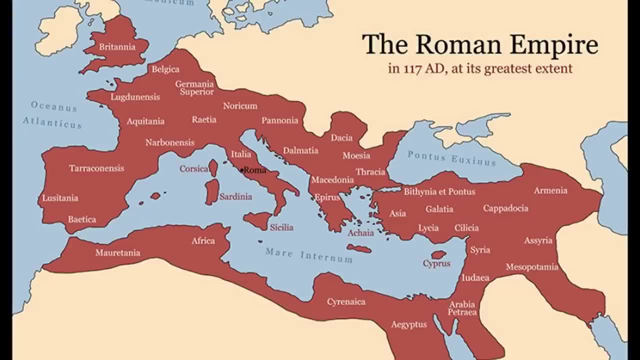 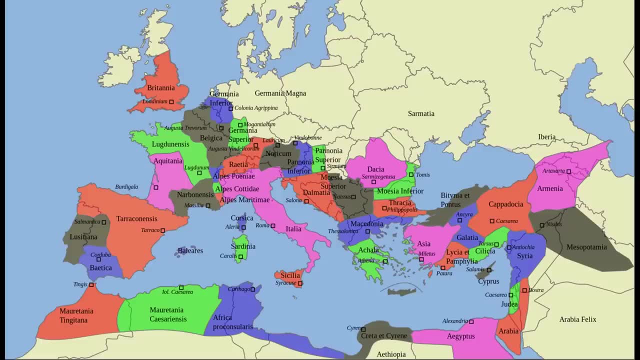 With the Caesars controlling approximately one in four people on Earth. during its height nearly 2,000 years ago. This included most all of modern-day Europe, the Mediterranean, North Africa and various places throughout the Mideast- A vast area especially for ancient times. 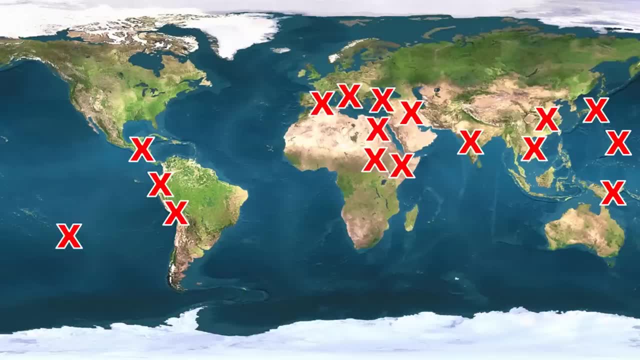 I show you this map because, for the rest of the video, I'm going to show you dozens and dozens of striking similarities from civilizations that are not supposed to have had any contact or connection to each other at all, Having been separated by oceans and continents. 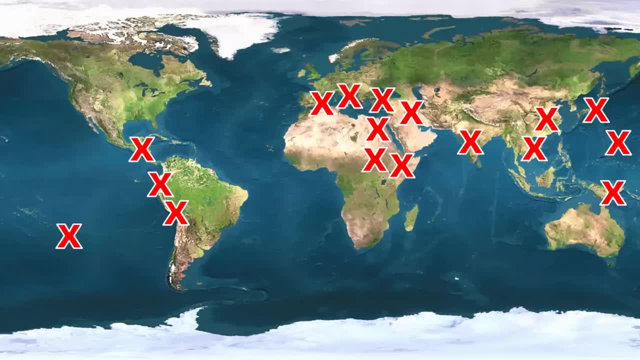 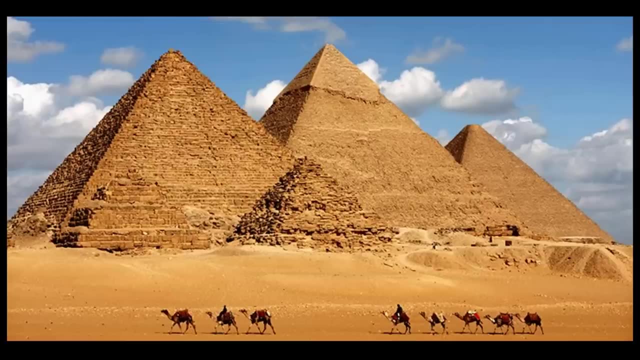 So, with that said, here we go. Perhaps one of the first things that comes to mind when we hear the word ancient ruins are the pyramids. Yet many people are not aware that pyramids have been found throughout five continents around the world. 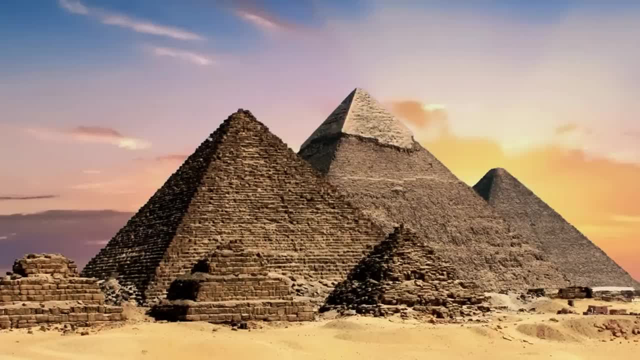 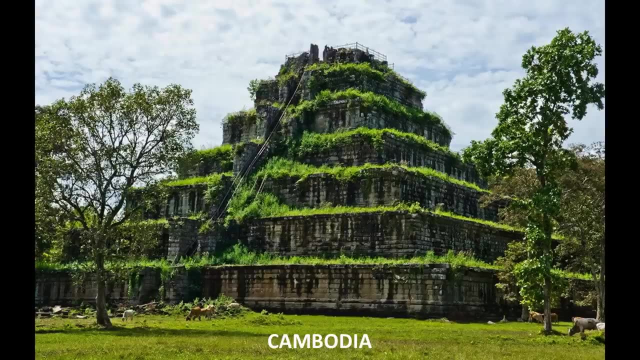 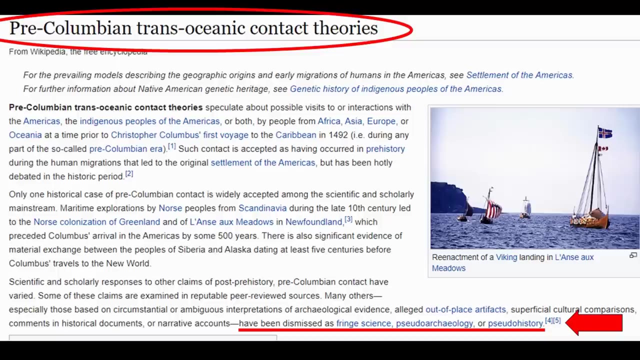 Although most everyone, surely, is familiar with not only the Egyptian pyramids but the pyramids of Central America as well, along with various pyramids within Southeast Asia and the country of Cambodia. But let me be clear. It is firmly stated and taught in the world of academics, historians and archaeologists. 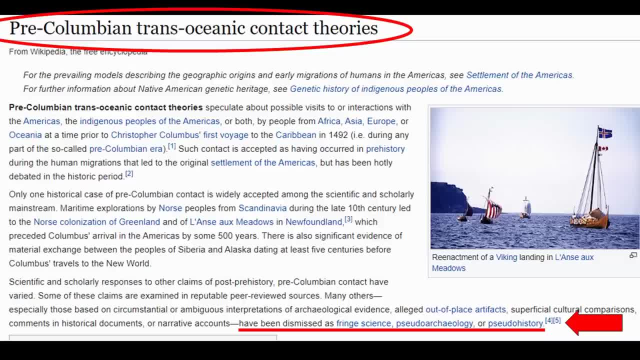 that there is no connection between Ancient Egypt, Cambodia or Central America. so enough toÉ America. In fact, it is considered to be, and I quote "fringe science, pseudo-history and pseudo-archaeology to suggest that it was possible for these. 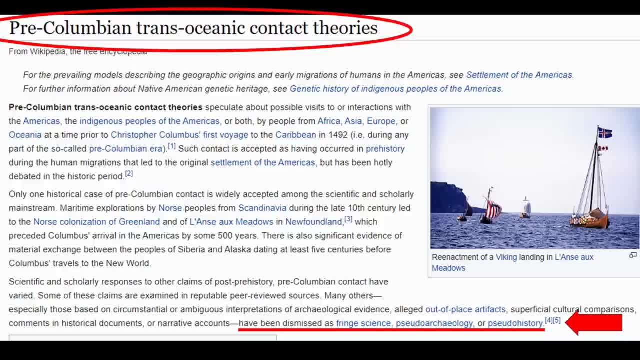 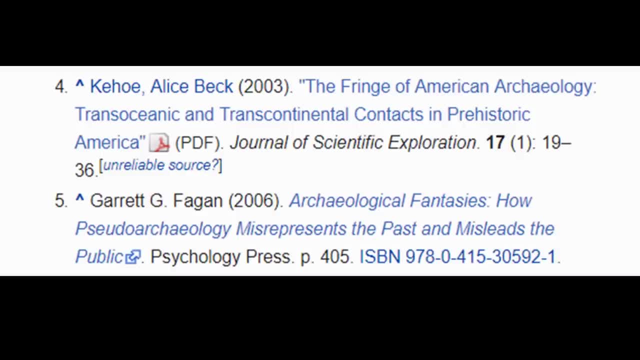 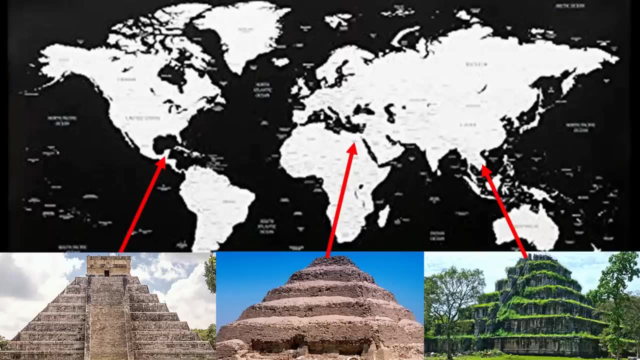 ancient civilizations to have been connected across the oceans and the continents". In fact there have been many books and scientific journals written expressing just that. But let's take a second to compare the unique similarities between the Step Pyramids of Egypt, the Step Pyramids of Central America and the Step Pyramids of Southeast Asia. 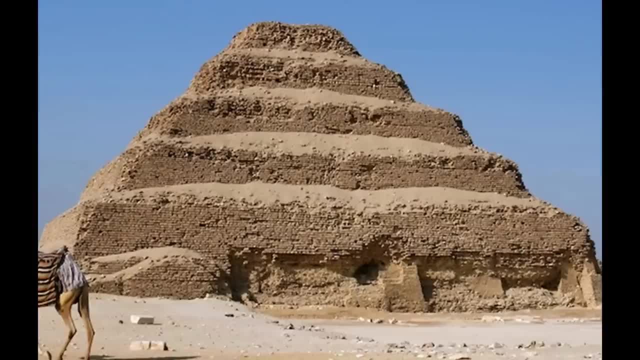 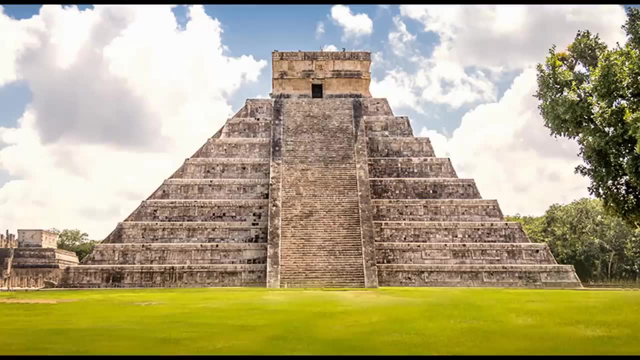 Archaeologists will tell you that the similarity is simply related to the primitive structural design of the pyramids themselves, and that you start with a larger foundation and make each additional layer smaller than the one below it. They go on to explain that this is the most simple structural design possible, and it's 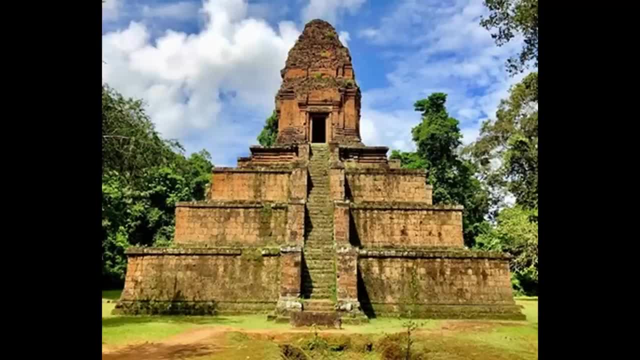 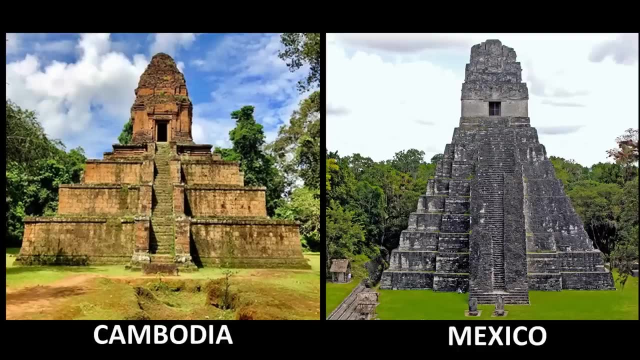 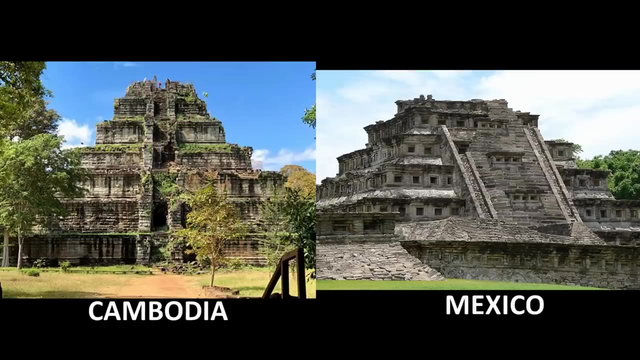 just a matter of natural evolution within varying civilizations to come up with this design on their own, again naturally and organically. I disagree, however. these pyramid similarities are not a main supporting argument for this video, but rather a start point. But I have to say that I do not think that these similarities are just a coincidence. 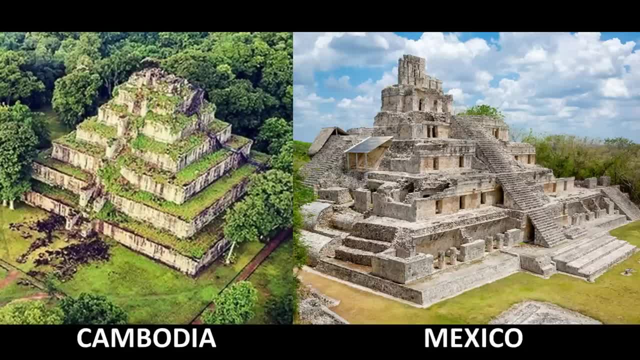 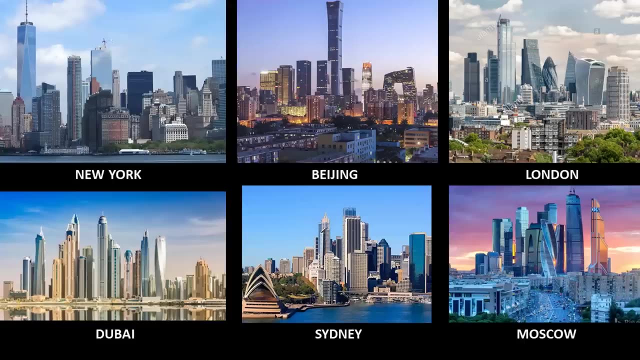 especially when you consider them from a side-by-side comparison. Look and think for yourself. Here's what I would argue: That although in today's world we are separated by oceans and continents, we are still a global civilization that is absolutely connected, Regardless of country borders and different governments, and in any corner of the earth. 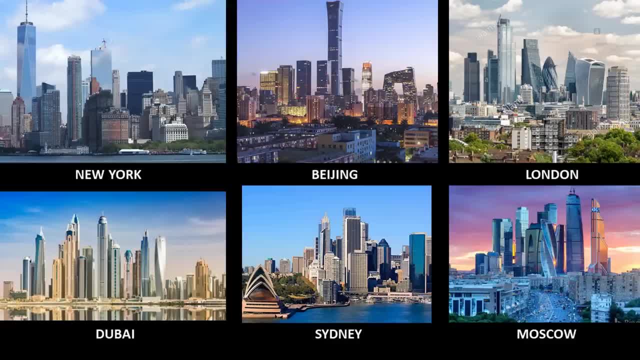 in any major city you will find skyscrapers And although they are all different from each other, they are still the same exact structural concept, made of steel, concrete and glass. Different in architecture, yes, but essentially the same nonetheless. 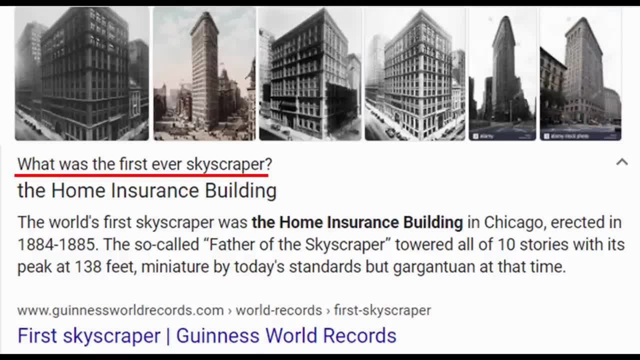 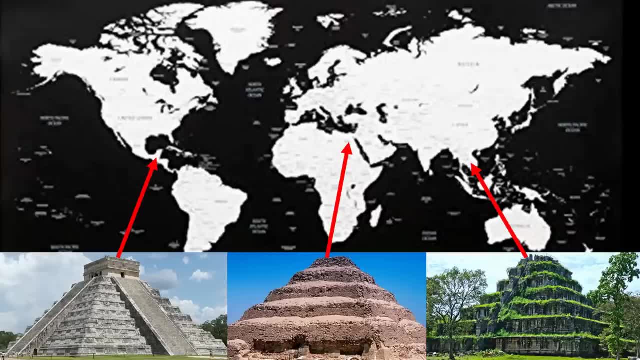 In fact, the very first skyscraper started somewhere which happens to be in Chicago. From there, the concept spread across the world. It is my opinion that the same thing likely happened with the pyramids, And when you see what else I have to share with you in this video, you'll understand. 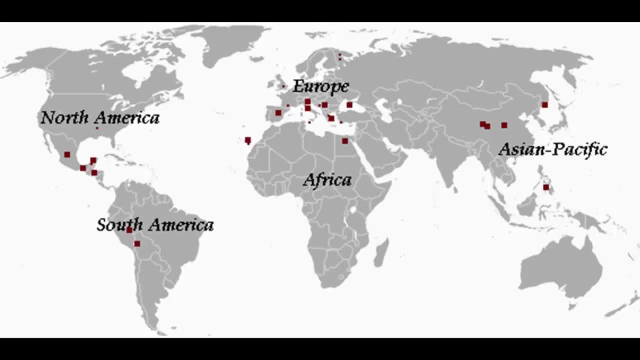 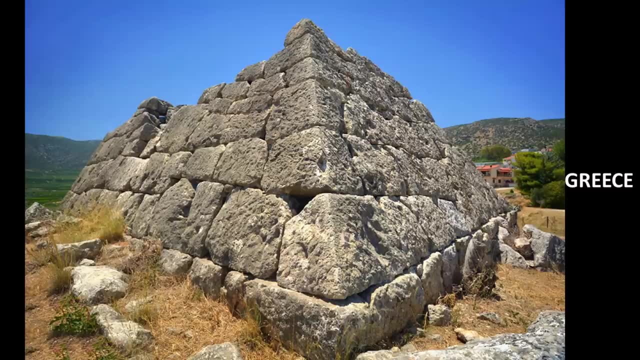 why, And like I mentioned a few moments ago, pyramids are found across five continents around the world, And one place that I know most people never knew of is Greece. Look at this here. and although much smaller compared to other pyramids around the world, 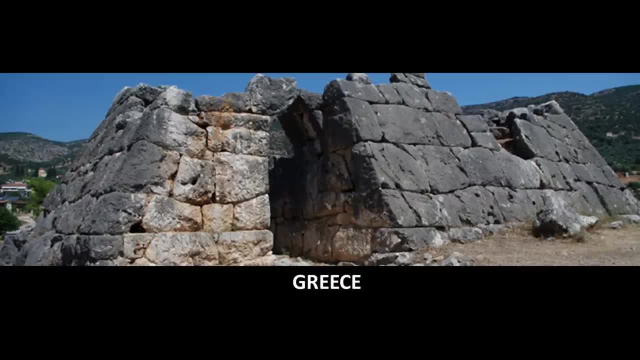 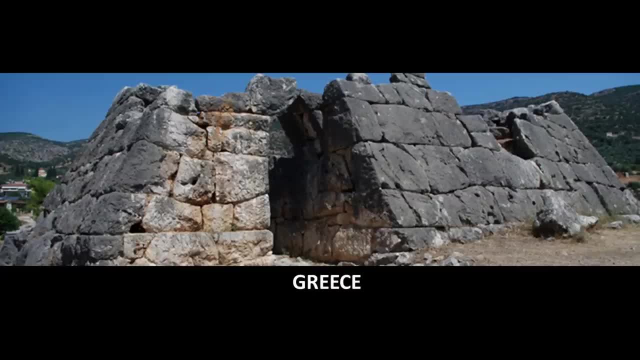 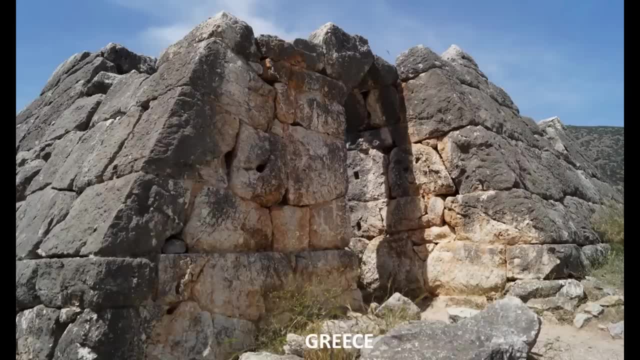 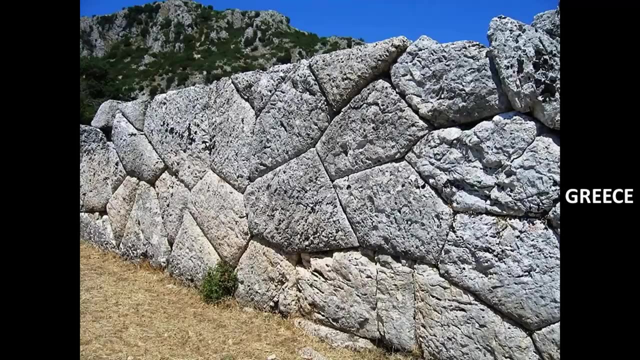 I wonder how many people watching this video had never seen or heard of this Greek Pyramid before, particularly people living outside of Europe and the Mediterranean. Something that you may not be aware of involving ancient Greek is that they have polygonal stone walls around the world waar they do not have this kind of associations. 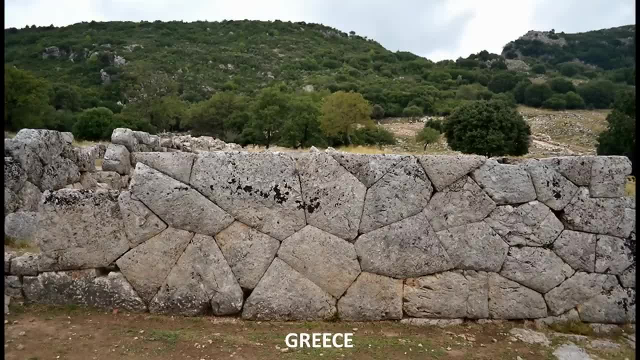 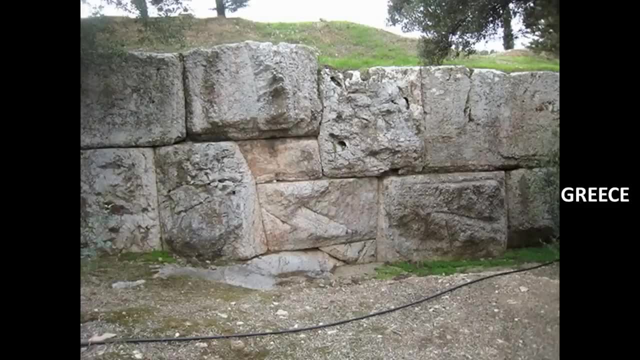 Should these always exist or not? Well, don't follow my data. the country They've survived thousands of years and some of the worst earthquakes in human history. Most people are not aware that Greece has polygonal walls. as you won't find this. 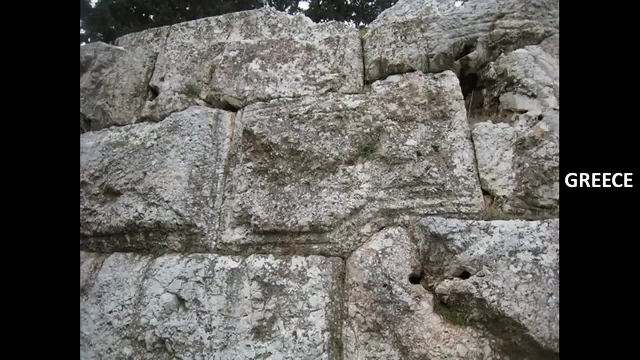 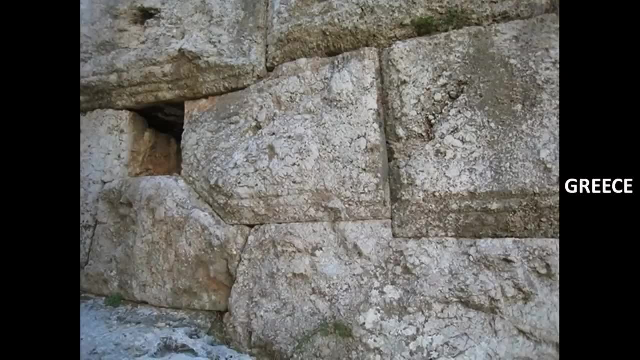 structure designed in and around Athens where all the other notable ancient Greek ruins are found and visited. And besides that, when we typically think of or hear of ancient polygonal stone walls, the ruins of South America and the country of Peru likely come to mind, which I'll 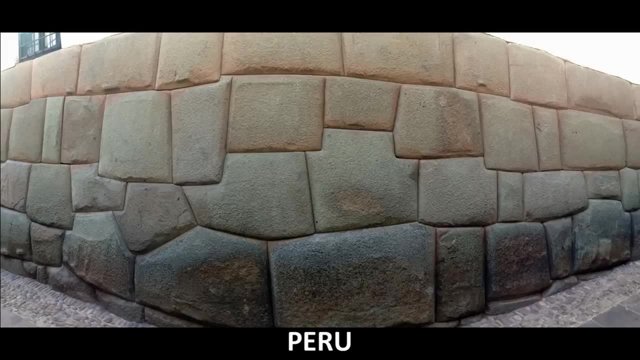 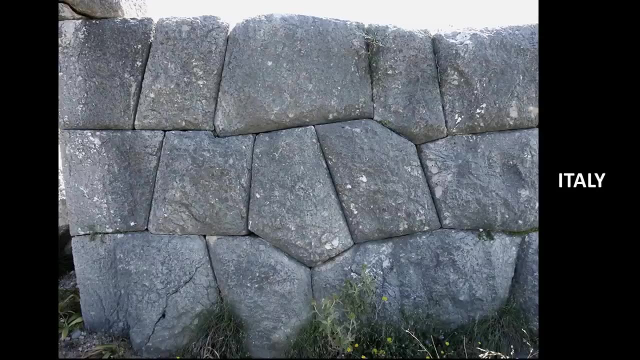 be discussing more of in a moment. but just like the little-known stone walls in certain places in Greece, there are also a few examples in Italy as well, Again, something most people do not realize, as you won't find an abundance of this type of ancient stone structure in and around Rome either. 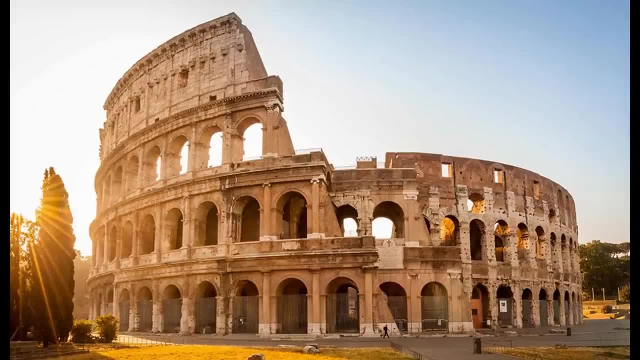 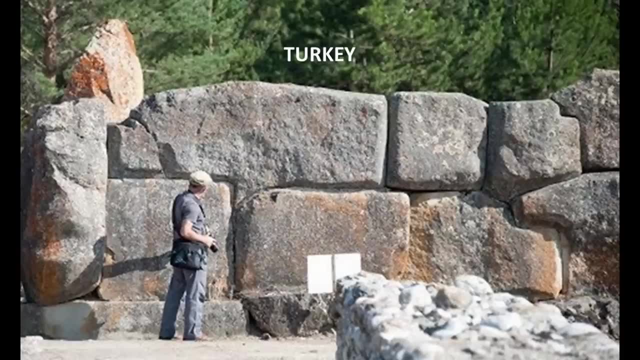 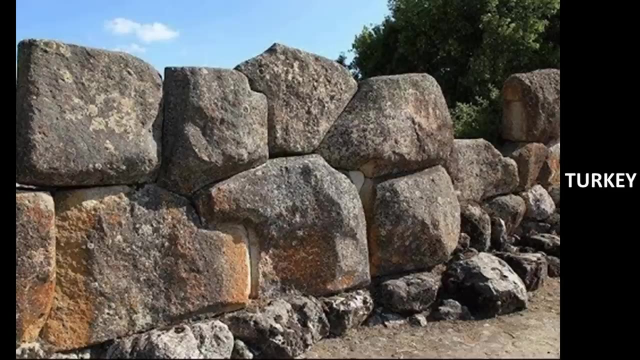 and all the other Roman tourist attractions take attention away, just like in Greece. It's also worth mentioning that there are incredible and massive polygonal stone walls in various places in Turkey as well. Take a look at the these and again be reminded of the massive stone walls in Peru- Definitely not exactly the same. 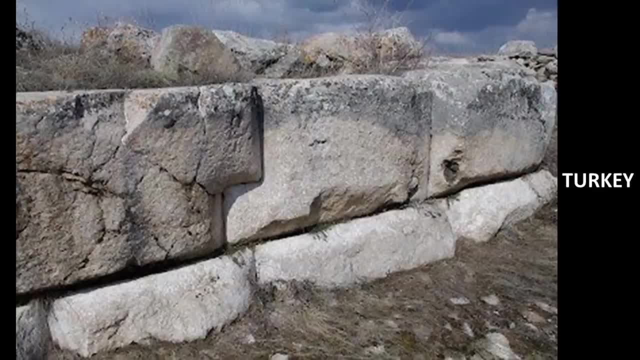 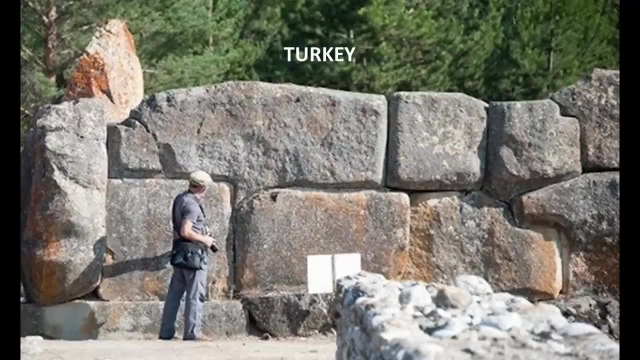 but the concept sure is, and it's unbelievably difficult of an undertaking to accomplish. But that aside, and although these are certainly credited to the Greeks and Romans, we have to ask ourselves why we find something so strikingly similar all the way over in Peru. 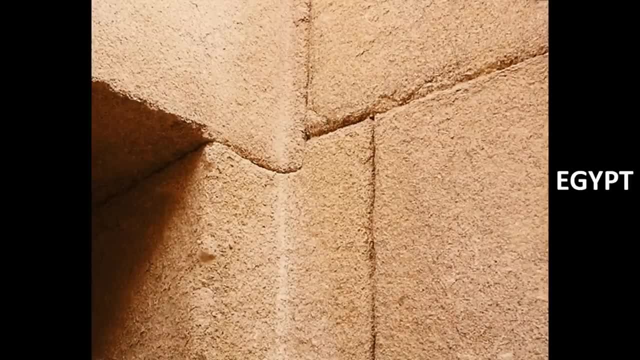 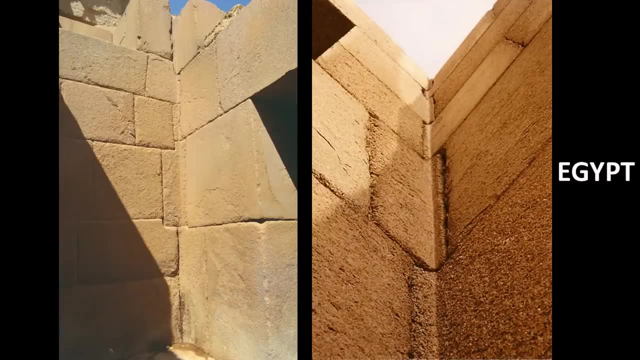 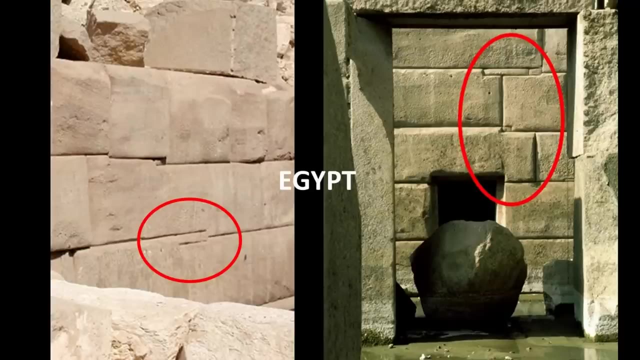 Not only that, we find similar examples within ancient Egypt as well. This raises questions because, as far as we were taught, there can be no possible connection between the ancient cultures of South America and Egypt, or to that of Greece and Italy. However, what I'm about to show you next, 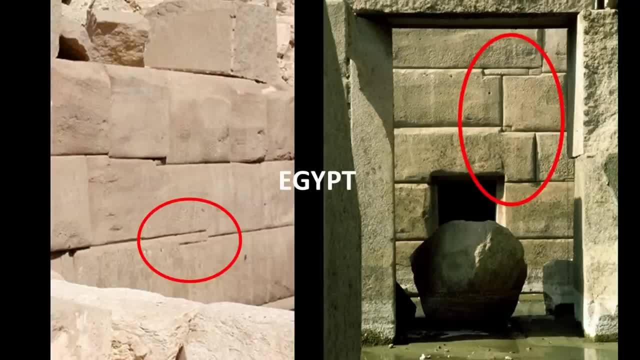 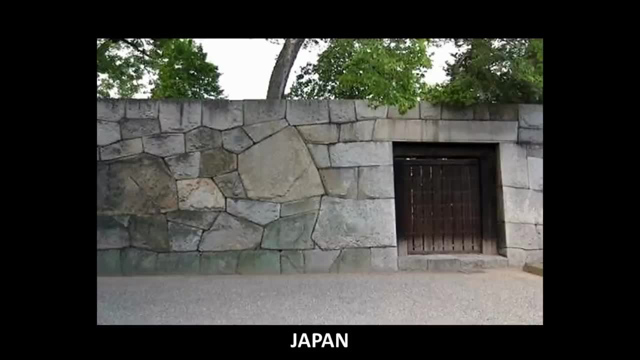 may take you by surprise, as there are several examples of incredible ancient polygonal stone walls all the way over in the island country of Japan. Leave a comment if you are completely unaware of these walls and, like I said, there are a variety of different examples of them. 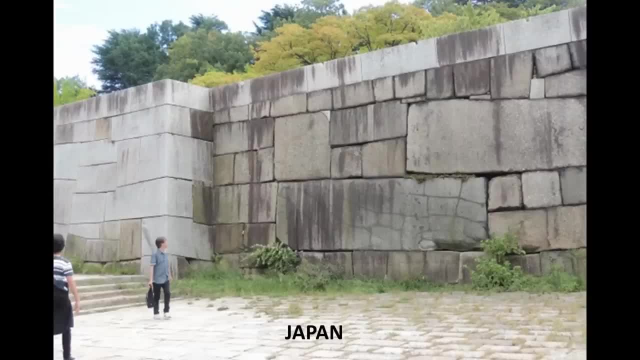 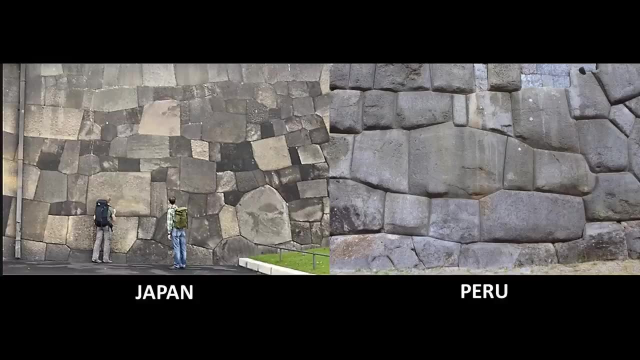 and I'm only showing you a few here in this video. Compare it to the stone walls of South America which, although is not exactly the same, they really remind you of my skyscraper analogy I gave moments ago. Is this really just a coincidence or a simple matter of organic human ingenuity? 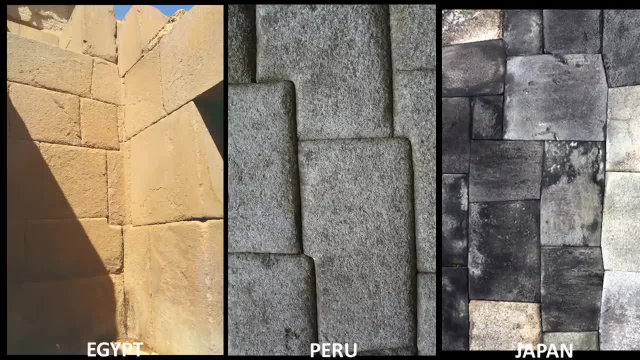 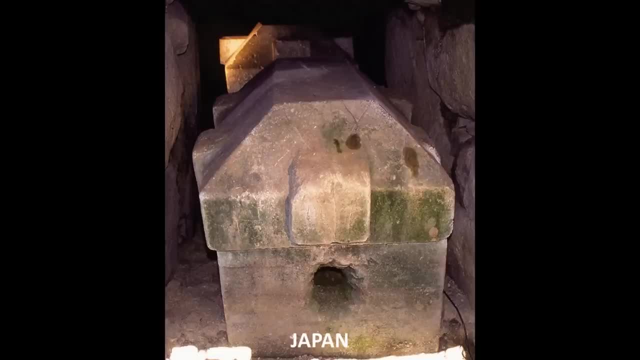 within different civilizations that are worlds apart. Well, if that's what you think, wait until what you see next. This is a stone box sarcophagus found in ancient Japan. Now compare it to a notable stone sarcophagus that made headlines. 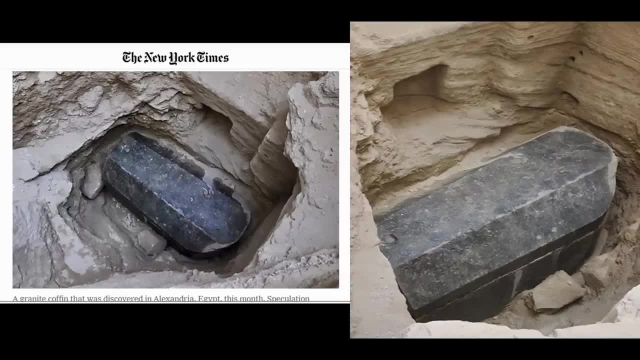 around the world in 2018 upon its discovery, with the whole world waiting in anticipation for it to be opened so we could see what's inside. I made two videos on this, if you're interested, but look at the design of the stone lid and now compare to the stone lid found in Japan. 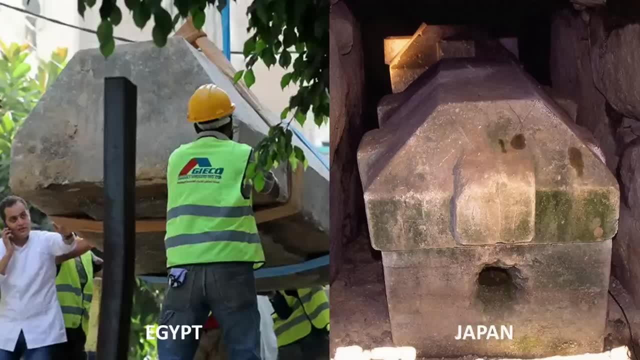 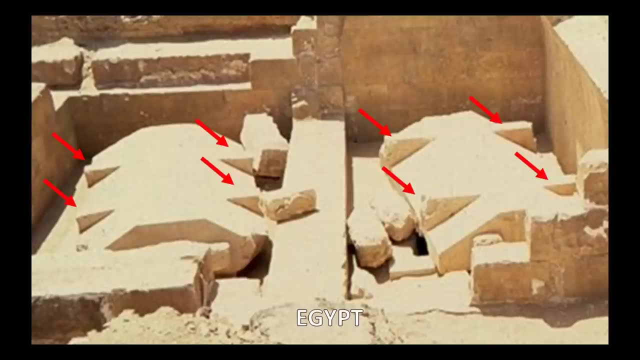 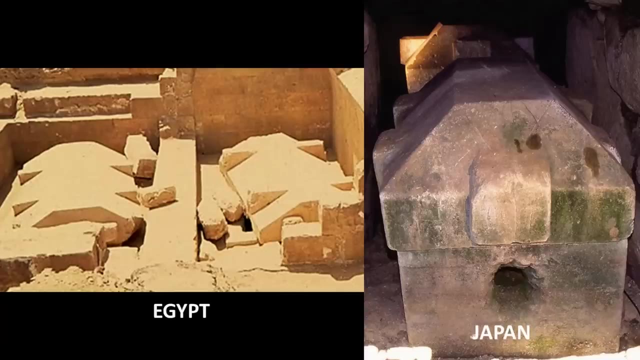 both having somewhat of a triangular shape, although not exactly the same. However, now compare the Japanese stone lid to others that are found in ancient Egypt. Wow, Is this really just a coincidence? Look at this and think for yourself. I do not see a coincidence here. I see a connection. 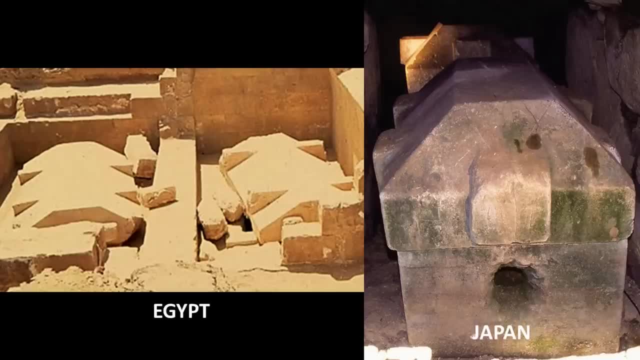 An ancient connection that's not supposed to be possible at all. I mean, we're talking Egypt and Japan, Worlds apart, especially in ancient times, and, of course, according to the textbooks, there is no connection at all Now, remember the Japanese polygonal stone walls I just shared with you. 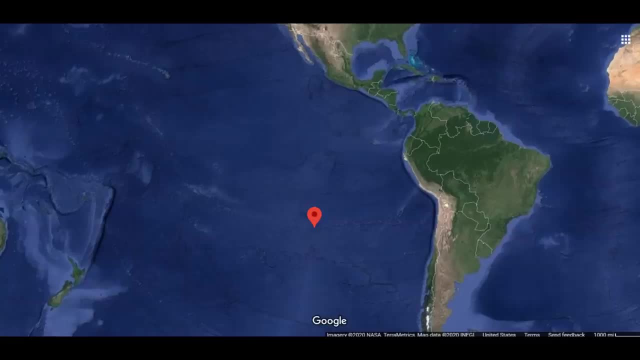 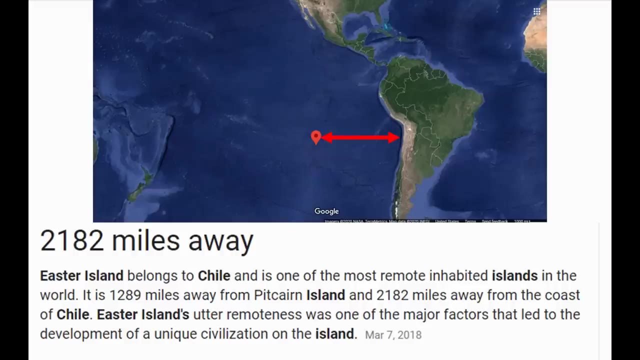 and let's head all the way to the complete opposite side of the Pacific Ocean, to remote East Asia. This is the eastern island, which is more than 2,000 miles from the nearest point of South America. Of course, when we think of Easter Island, the notable Moai statues are probably the first thing. 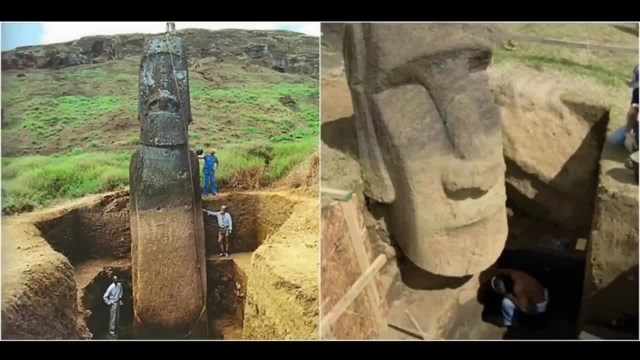 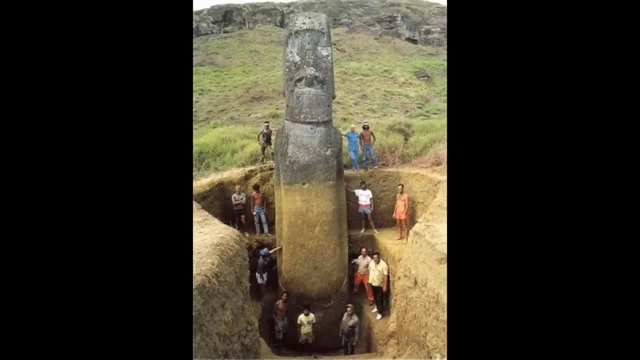 to come to mind. Many people are surprised when they learn just how massive many of them actually are once they've been dug up and excavated. Just look at that. However, what most of you are likely to find even more surprising is to learn that there is an example of a polygonal stone wall. 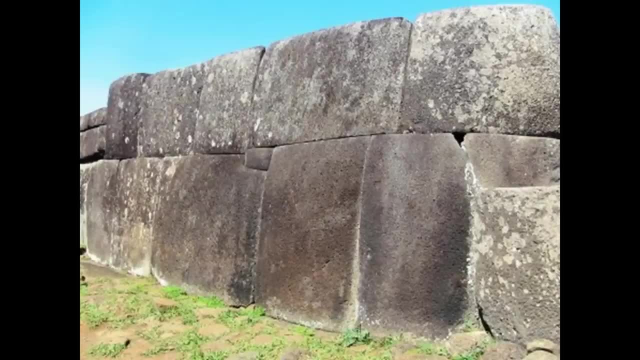 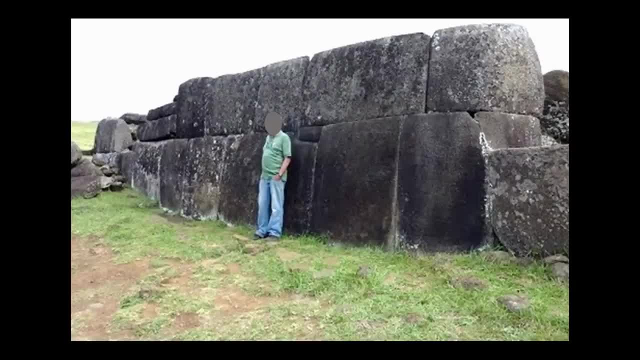 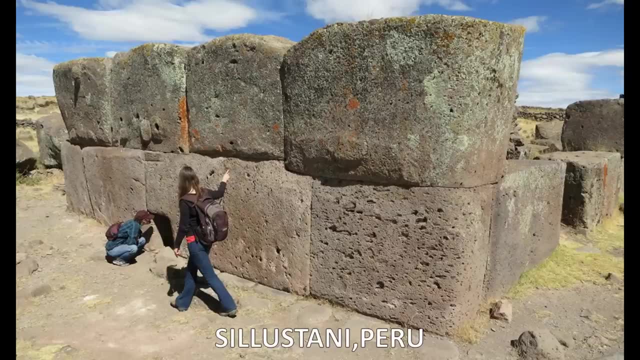 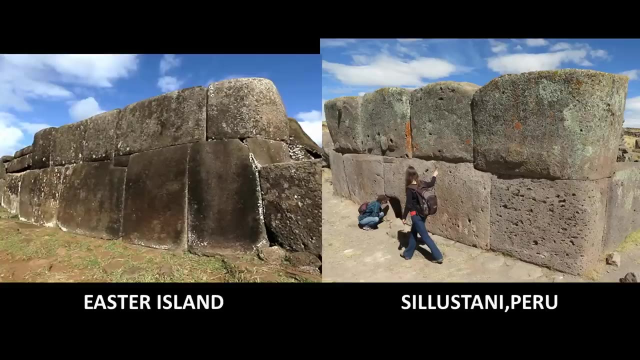 as it's the Moai statues that get all the attention. Now compare this wall to a wall all the way over in Peru. Look at these comparisons and tell me that this isn't a total match. The side-by-side comparisons definitely make my eyebrow go up, because the consensus of academic 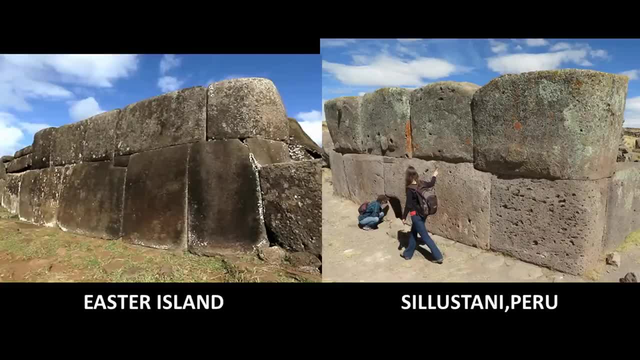 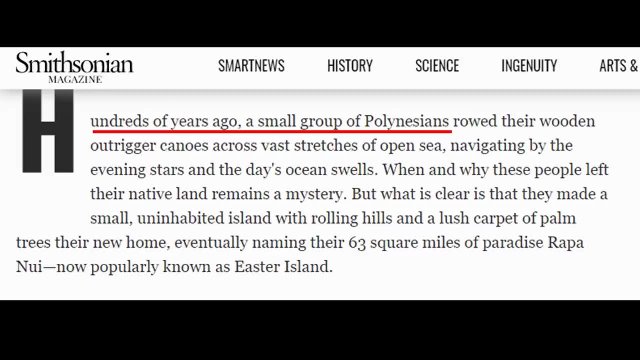 scholars is that there is no connection between Easter Island and Peru. It is also widely accepted that the people of Easter Island came from the Polynesian Islands to the west and settled on Easter Island. I do not disagree with that at all. However, let me quickly remind you of something. 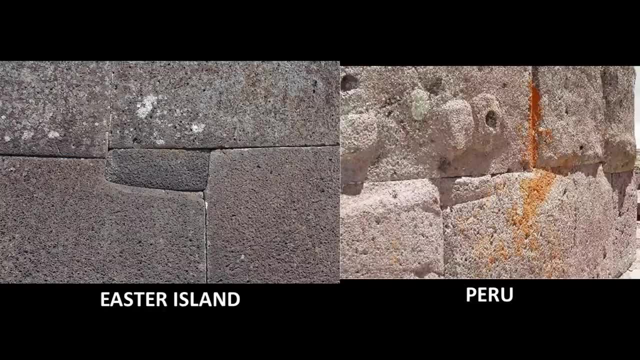 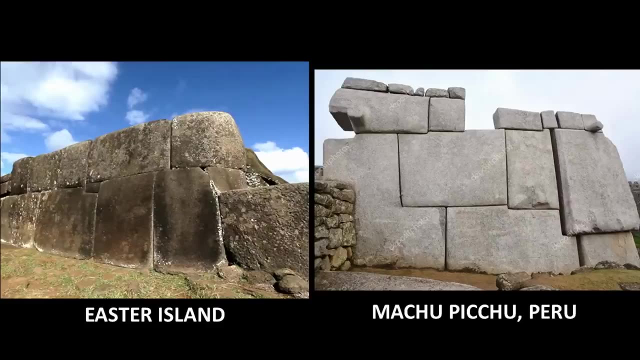 before I show you something else, which is that trans-oceanic sea travel during this time frame was considered to be impossible. and again to suggest it is fringe and pseudo-archaeological. So how do we explain the unbelievably similar comparison to the little-known cloud people? 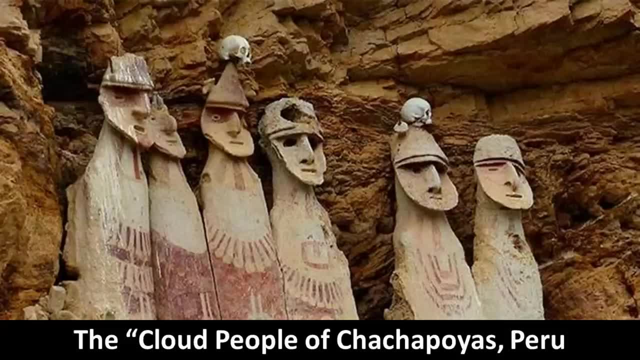 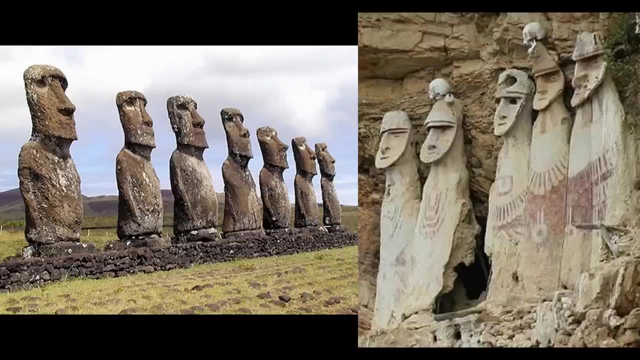 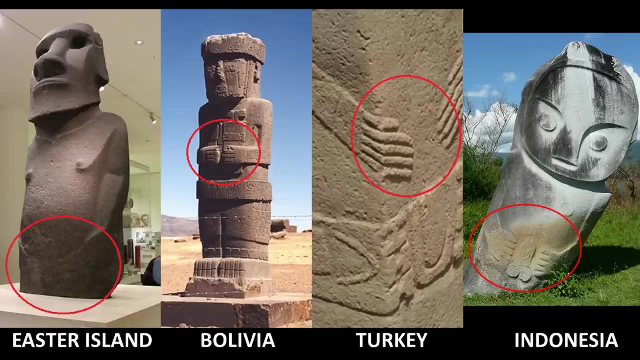 statues of Peru. Tell me this isn't unbelievably similar and again created at a time when travel between Peru and Easter was not considered a possibility. But that's not all. Compare these statues to others as far away as Turkey and get this Indonesia, Although not exactly the same. 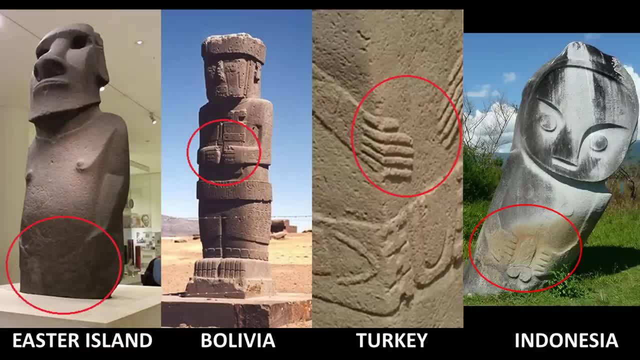 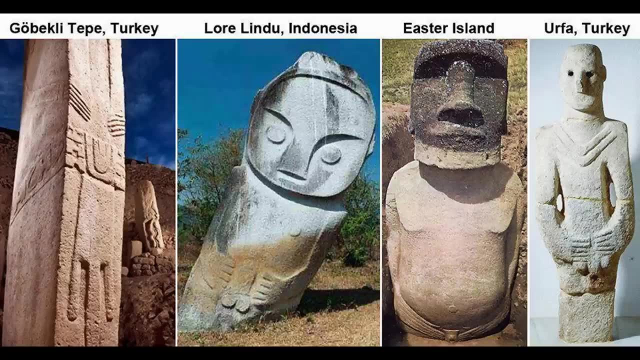 when you look at the more nuanced details, such as hand positions and unique facial and jaw structure, I mean: come on, is this also just a coincidence? And then we remind you that the site in Turkey you see here, Gobekli Tepe, is the world's oldest megalithic site on earth, dating back closer to 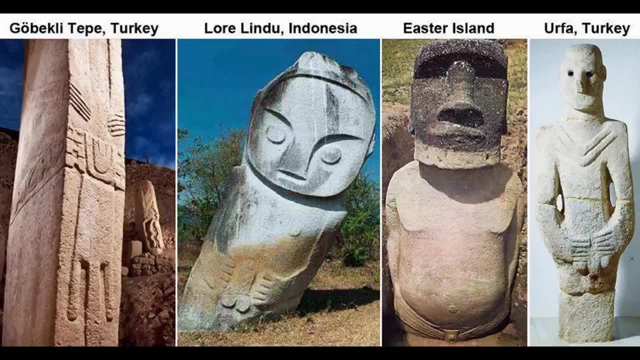 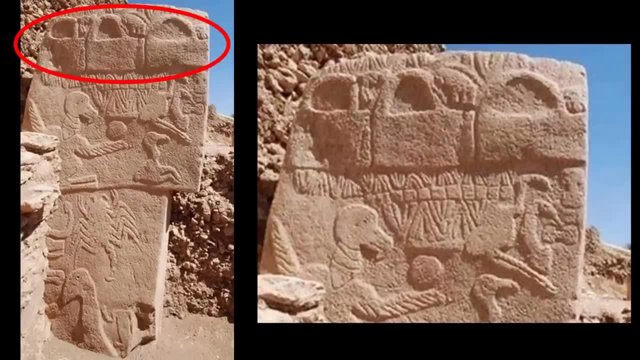 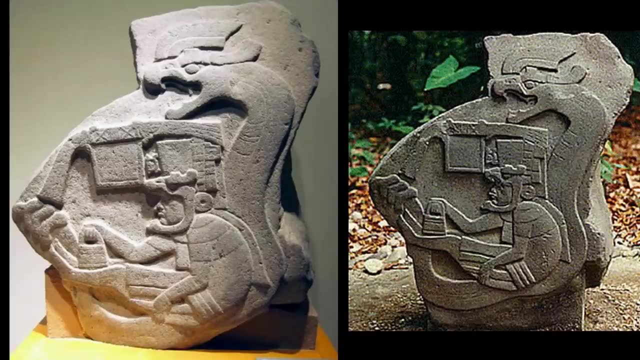 12,000 years and was buried up until excavations began in just the 1990s. Something you'll find at this same site is the specific stone carving of someone holding a handbag. This is a very unique and specific connection that you will also find all the way back in Mesoamerica. 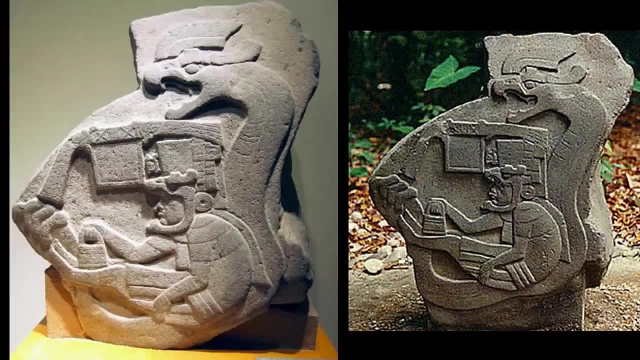 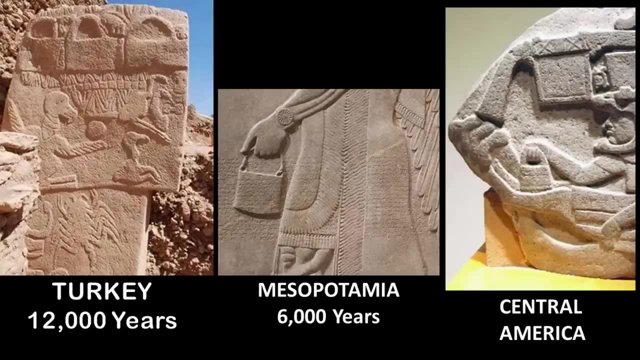 among the Olmec culture. This is so unbelievably similar. and to think that the bags themselves, the stone carving, dates back 6,000 years earlier from our first known documented civilization, which is the Sumerians, which they themselves have depictions. 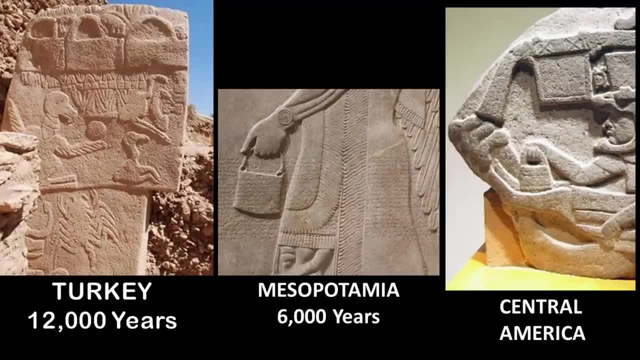 holding this bag and they are 6,000 years older than we are from present day right now. Incredible. How can something so unique be just a coincidence? However, that's what science, community of academics and archaeologists say about it. Yet most people walking around society have never. even heard of this before. However, that's what science community of academics and archaeologists say about it. Yet most people walking around society have never even heard of this before. However, that's what science community of academics and archaeologists say about it. Yet most people walking around society have never even heard of this before. 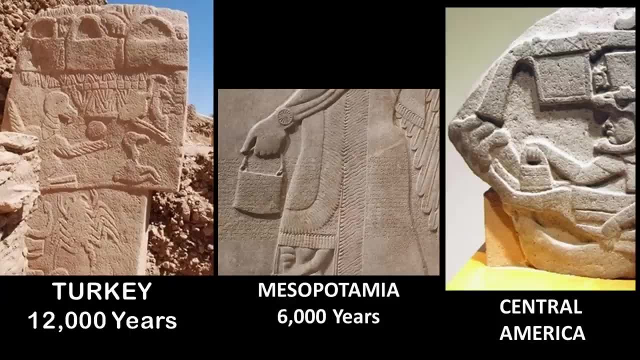 The authorities in the academic world shun it. yet they never even shared it with you, so you could think for yourself. So what do you think about it, having seen about these handbags for yourself? Is it just a coincidence? Now, speaking of the Sumerians, it's also worth mentioning that they 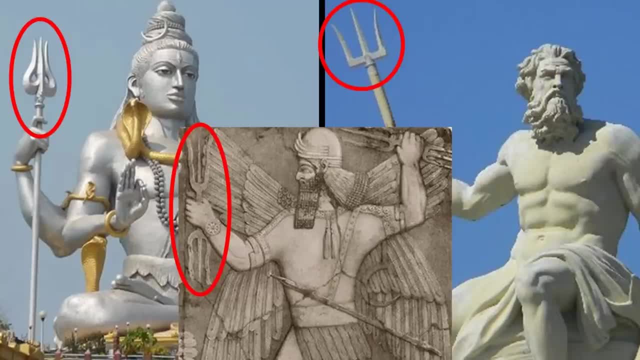 share another similarity to that of ancient Greeks and Hindu gods of ancient India, which is the depiction of the trident. But does this prove a connection? Well, by itself, no, But that is not the only similarity shared between the Sumerians and the ancient Greeks, The Sumerians and the archaeologists. 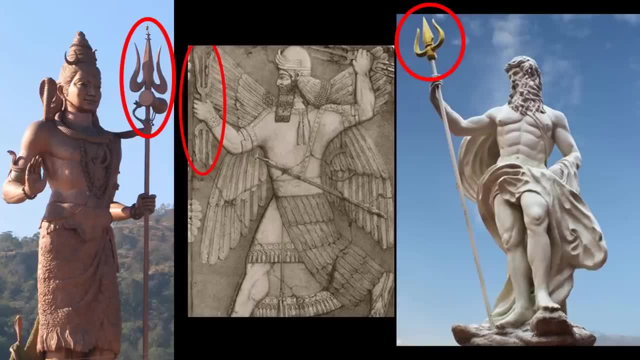 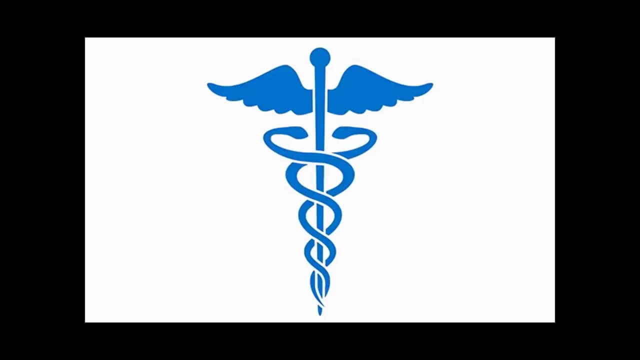 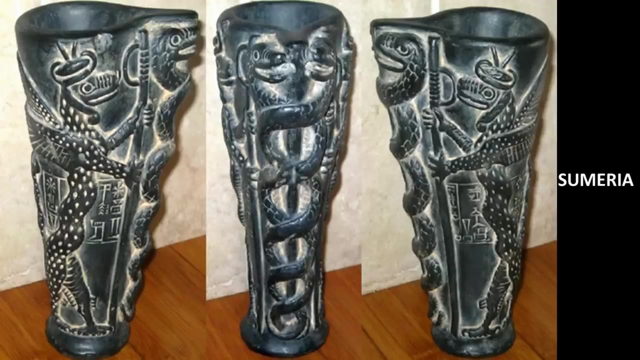 shared that the trident is the symbol of the two snakes, intertwined and found throughout the modern world today among the medical and healthcare industries. What most people do not know is that it has been found dating back as far as the ancient Sumerians of 6,000 years ago, like I just 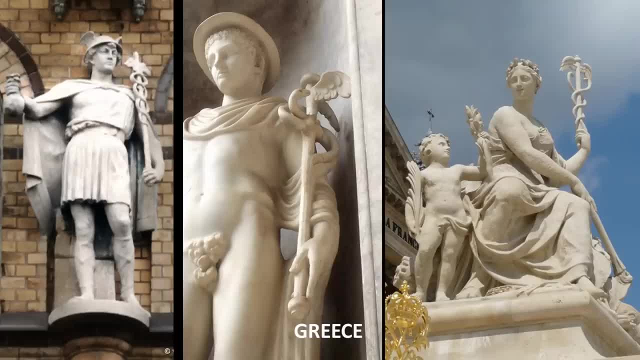 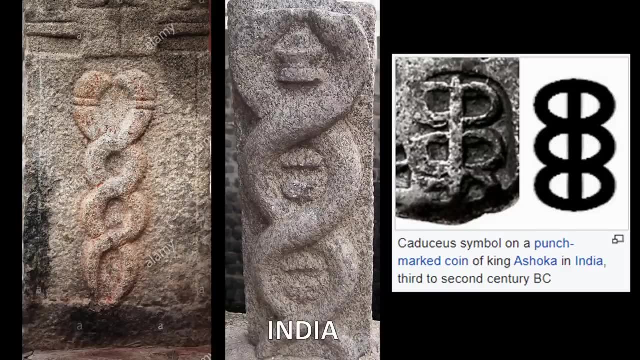 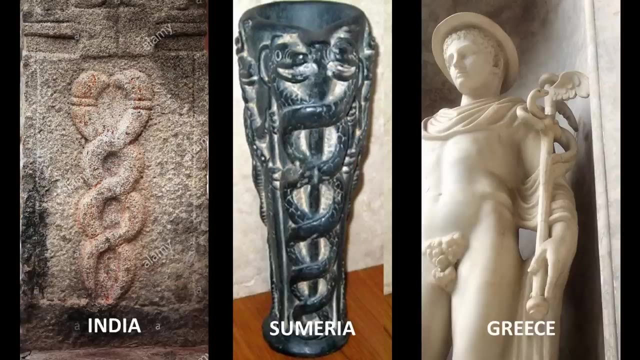 mentioned. Well, you may find it interesting to learn that this symbol was also utilized by the ancient Greeks as well, as in ancient India. Again, another interesting and specific coincidence for three separate cultures, separated by time and distance. But it does not stop there. 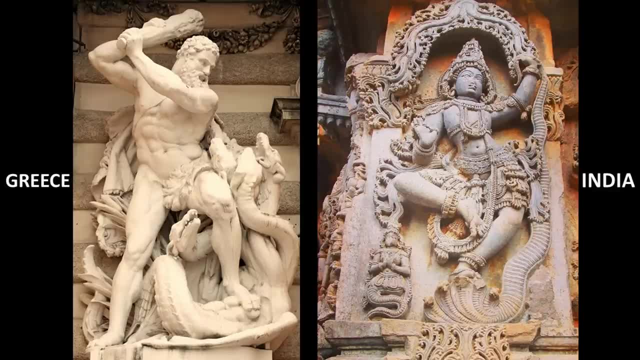 Even look at the depiction of a Greek god and Hindu god battling a multi-headed snake. Now that is a very specific and exclusive similarity, But again, by itself it is not earth-shattering. Although Greece and India are far apart, the ancient borders of the Greek empire 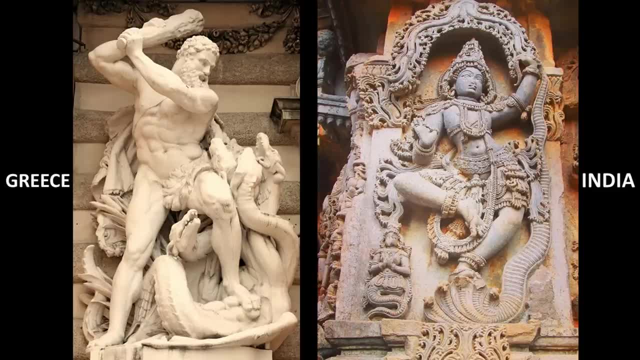 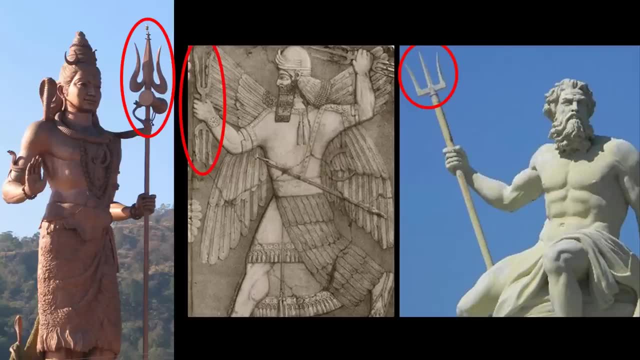 were once not so far away from India during the height of their civilization. But you would think that one of the most important details would be shared in school and the textbooks as a possible link, as a vast majority of people out there have never seen or heard of these details before. 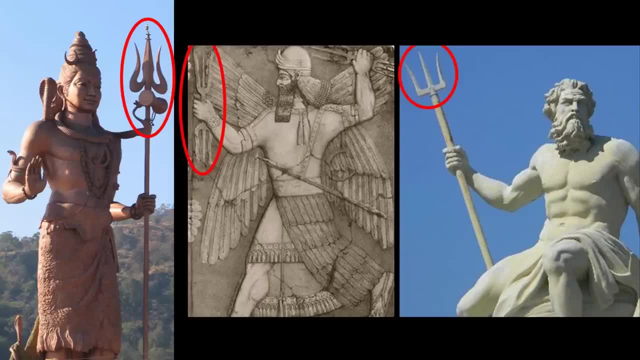 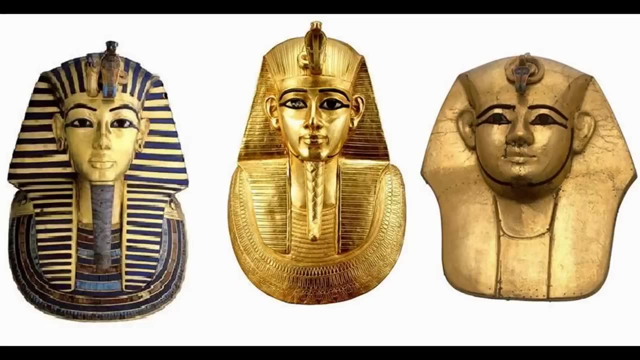 It seems to me that the ancient Greeks were more connected to India than is currently known or discussed. But let me keep going. I am sure everybody is familiar with the incredible gold funerary masks of the ancient Egyptians, But what's interesting is that this ties into a similarity of 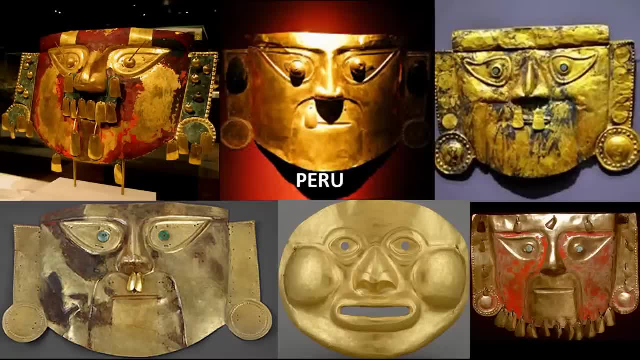 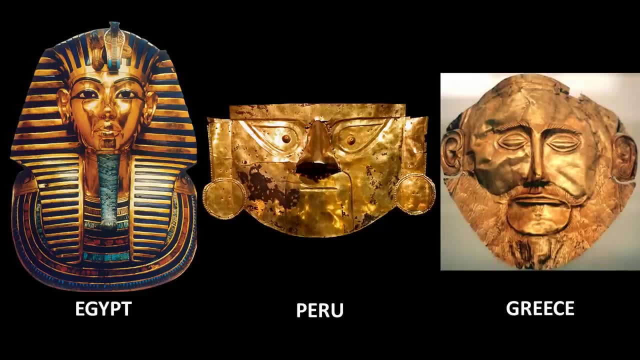 the Inca of Peru and South America, And that is a rare thing as well, as I only found one other culture that, and in only a few cases, also used gold funerary masks, And that was the Greeks, But only in the latter part of their 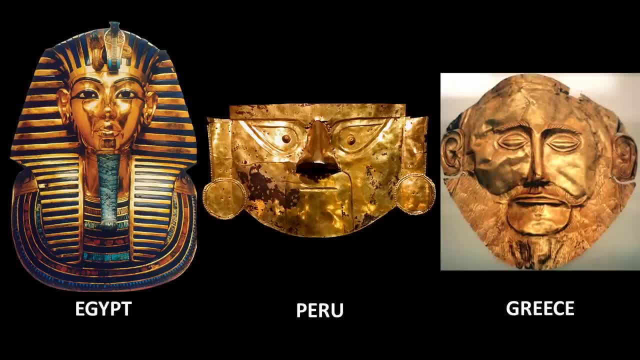 civilization. And you know, I have to say, isn't it amazing that the Egyptians were by far the best, the most highly skilled and sophisticated makers of these gold masks in comparison, And they did so thousands of years prior to the Inca or the Greeks. 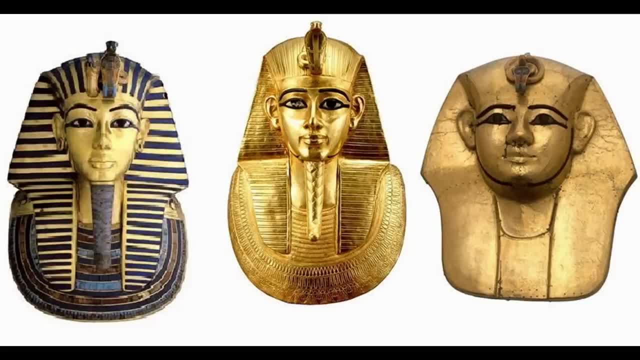 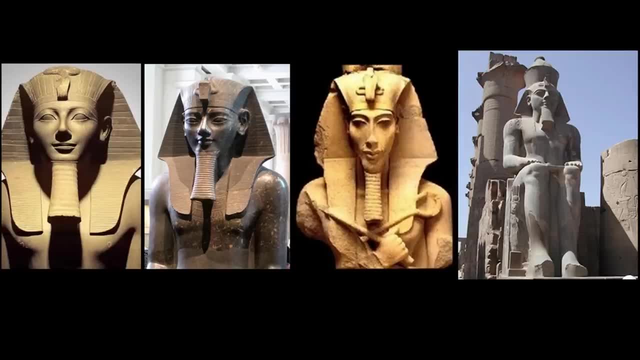 And speaking of gold masks, notice the depiction of a cobra snake at the forehead, something you'll also see on countless stone statues of pharaohs within ancient Egypt. Well, now take a look at how the cobra snake was depicted above the heads of ancient Hindu gods. 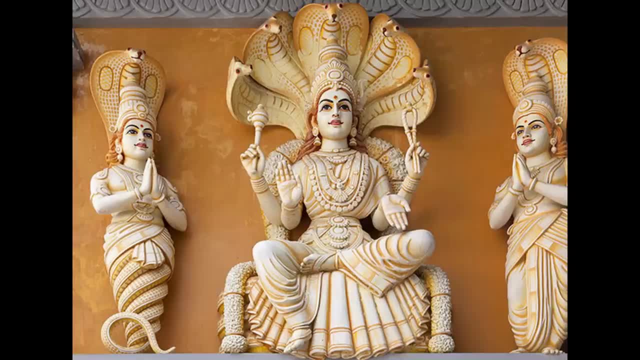 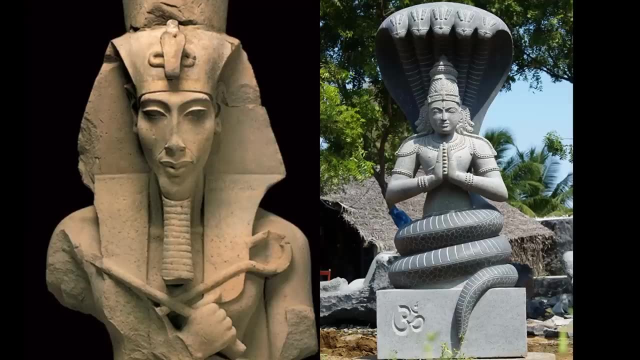 Here you can see just a few examples And although not exactly the same, this is without a doubt a specific similarity. I mean, why would anyone think to depict this a cobra snake at the head? Of course you can read the explanations provided by scholars. 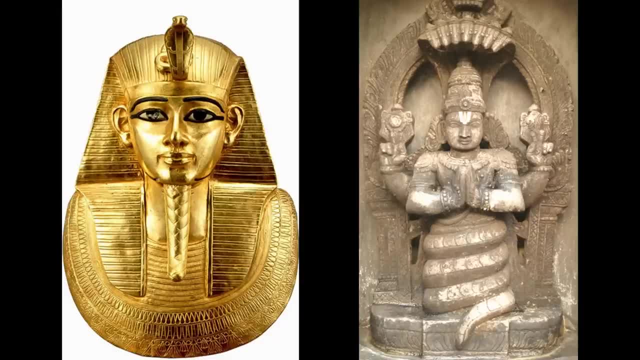 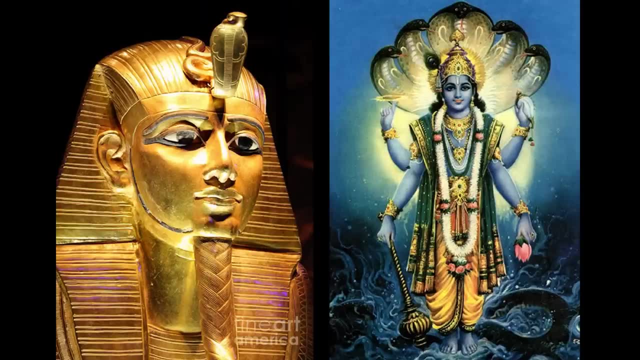 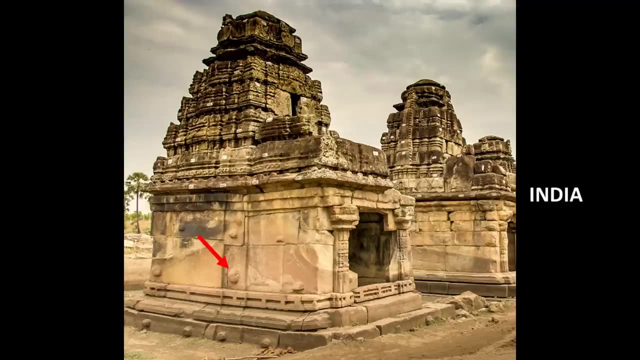 which is not consequential to this video, but rather the similarity itself, is the significance, Because there is absolutely no known, acknowledged connection between ancient Egypt and ancient India. But let me keep going. Now take a look at these examples of stone nubs on ancient sites in India. 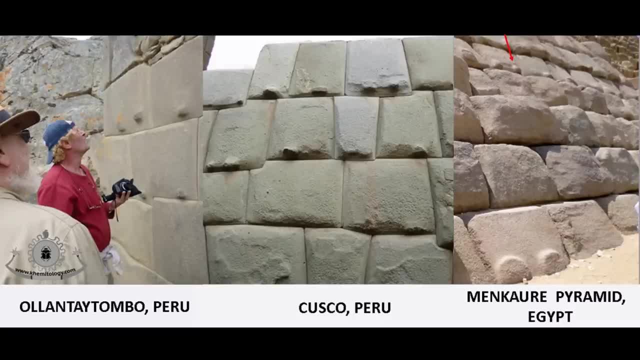 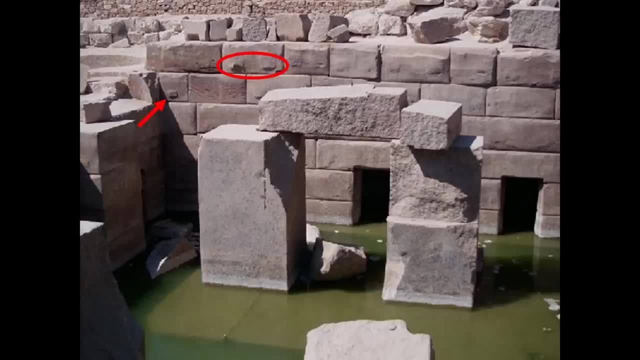 Many of you may have already heard me and others share examples of these unique stone nubs that are found in Peru and Egypt. Here are some examples found at Egyptian sites, including even that of a pyramid in Giza, as well as at the Assyrian as well, And this is just to show you a few examples. 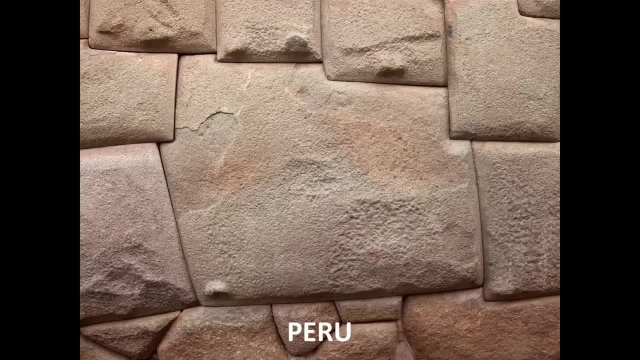 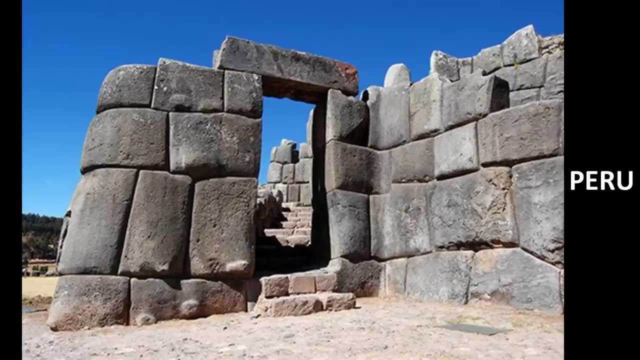 Now let me show you a few examples found in Peru, which there are many examples at various sites throughout this country, And let me point out real quick that I do not know the purpose of these nubs, but it is fair to say that it's not related to moving or lifting these stones as you would. first, 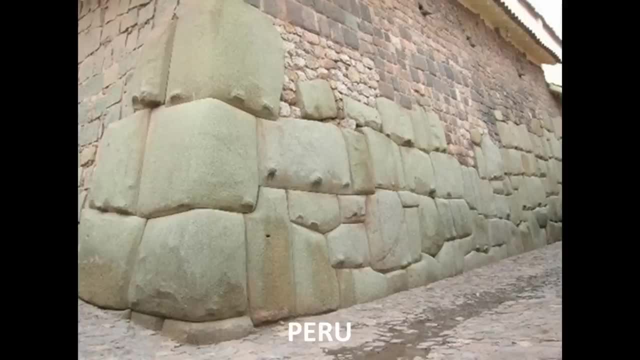 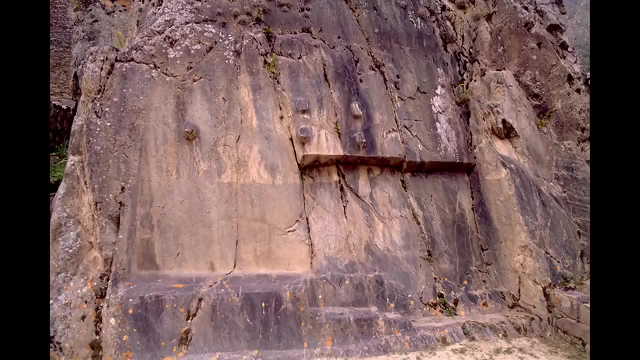 think, Because most of the stone blocks do not have them, Only some of them do. Plus, these nubs have various bedrock stones which obviously had no intention of being moved or lifted. Here are just a few examples to share what I mean by that. 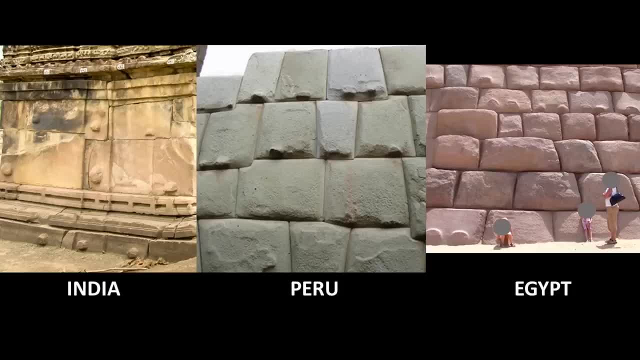 So, whatever their purpose was, it's not important to the point that I'm trying to make, although it's a fun discussion for another video. The point I'm making here is to show you the widespread global nature of these nubs. And let me say this real quick that even if the purpose of 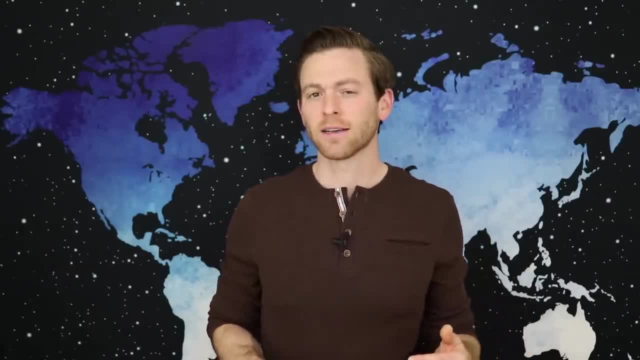 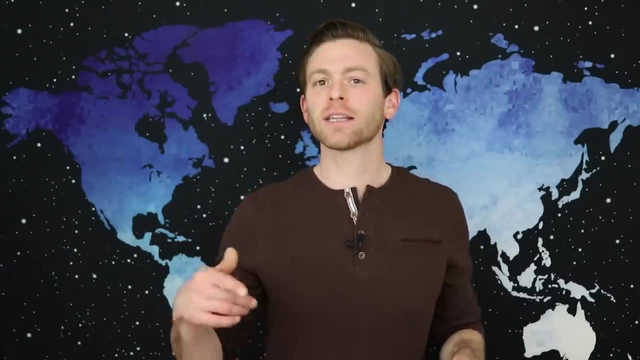 these stone nubs involved moving or lifting the stones themselves, then I would argue that it's even more supportive evidence of a widespread global connection. I mean, we have different ways of moving and lifting stones today and we are a global civilization that pretty much uses. 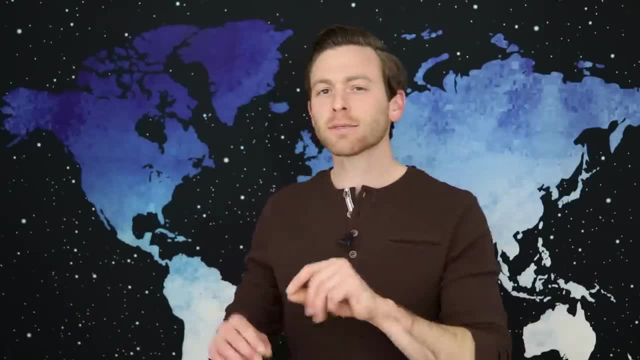 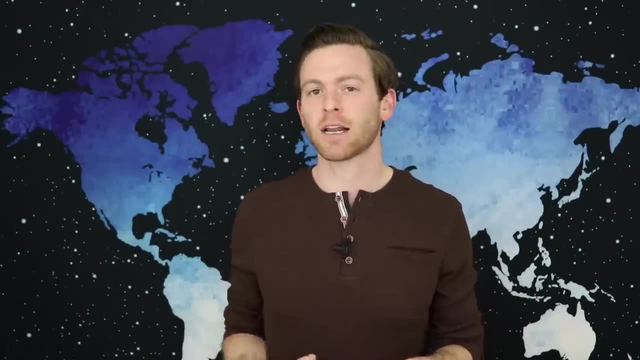 the same exact technology, right? So if there was some sort of purposeful stone mark on any stone that we're moving or lifting, that would be because we're using the same technology to do so. So if we find these stone nubs across the world, as you're about to see, 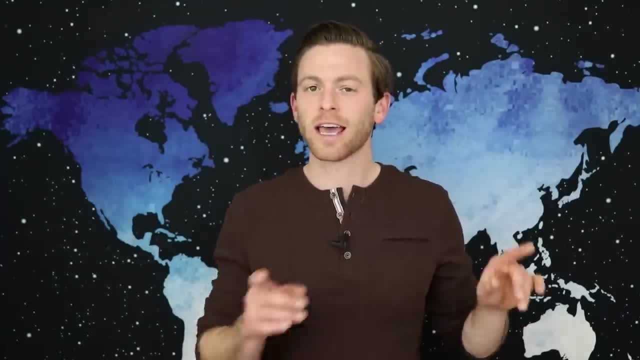 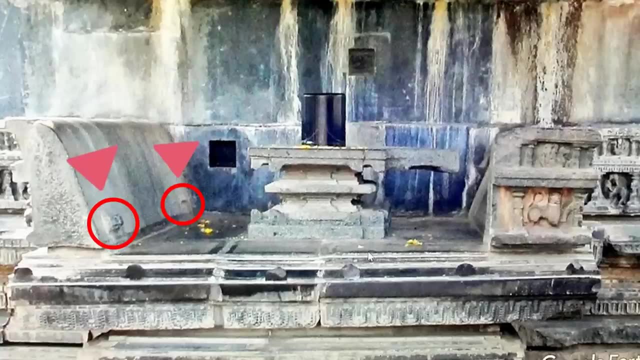 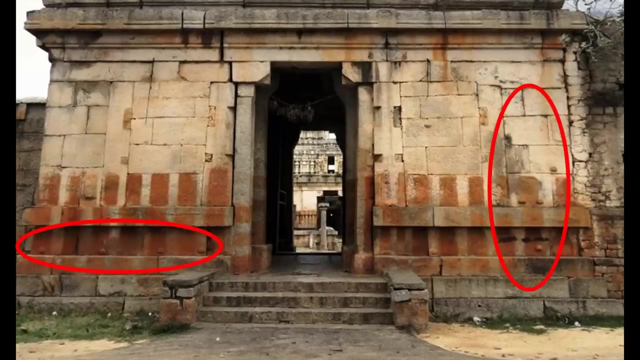 then you could argue that it's more supportive evidence that the ancients had a widespread, widespread global connection. But getting back to the widespread phenomena of the nubs, here are a few additional examples at various sites in India, And again, notice that they're on some, but not all, of the stones. I'll be curious to see comments. 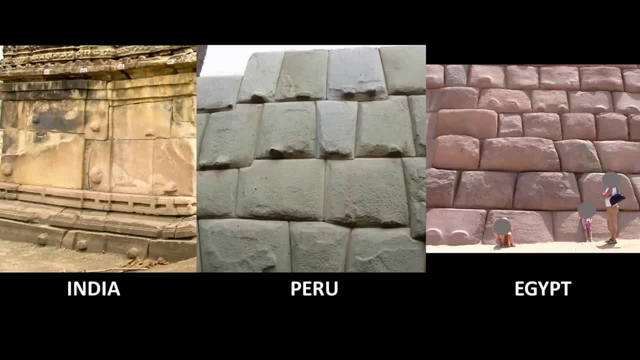 of how many people that were already aware of these nubs in Egypt and Peru who are only just now learning of these nubs being in India as well. Leave a comment if you are, But here's where it becomes even more thought-provoking, as these nubs are at. 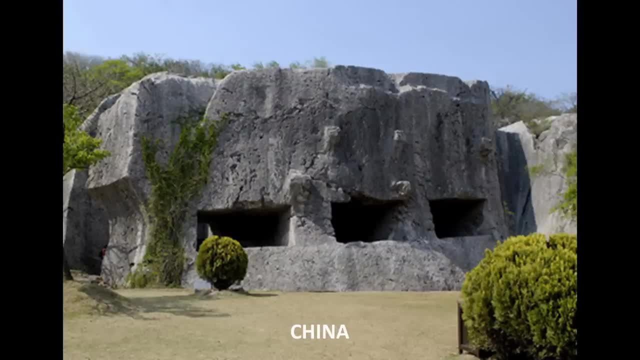 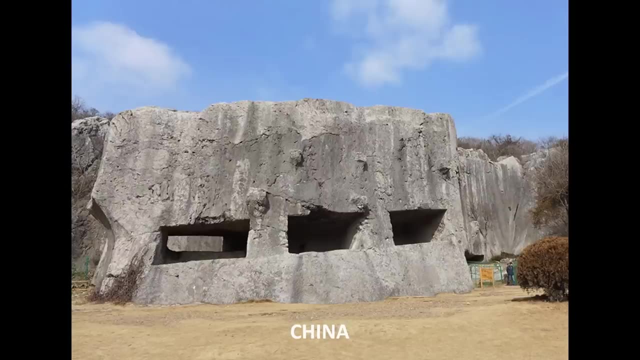 sites all over the world, For example, even at an ancient quarry in China. I'd be curious to know if there are other examples found at ancient sites in China, which is not easy to learn, as many sites are closed off to the public. Lame right. 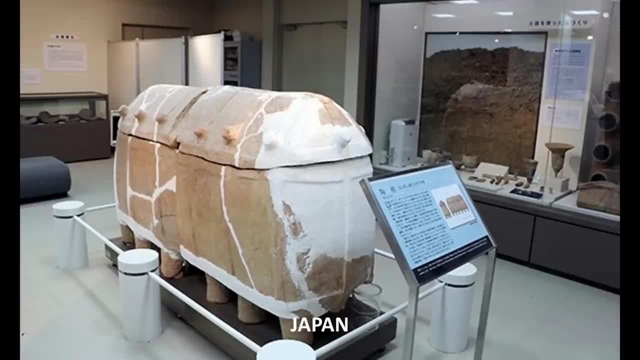 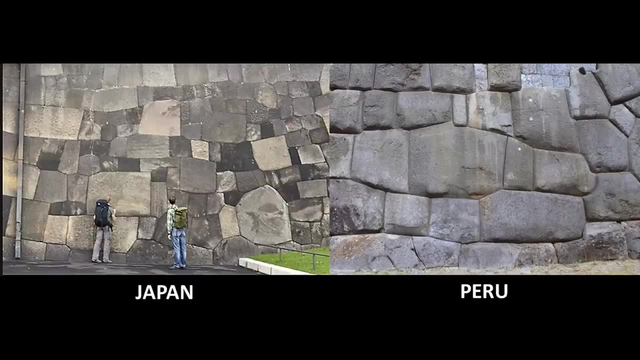 But you'll even find an example of nubs in Japan, which is interesting when you consider what I already pointed out involving the polygonal stone walls within Japan as well, and especially the comparison of the stone sarcophagus to the ones found in Egypt. 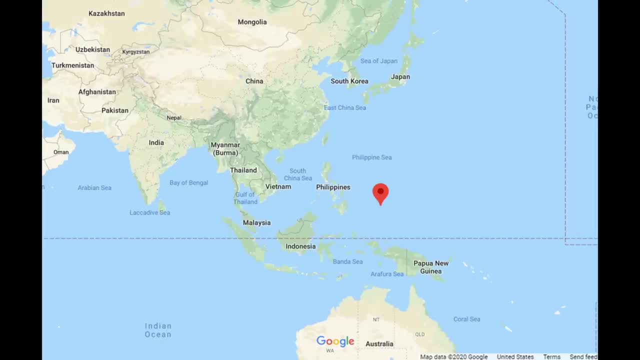 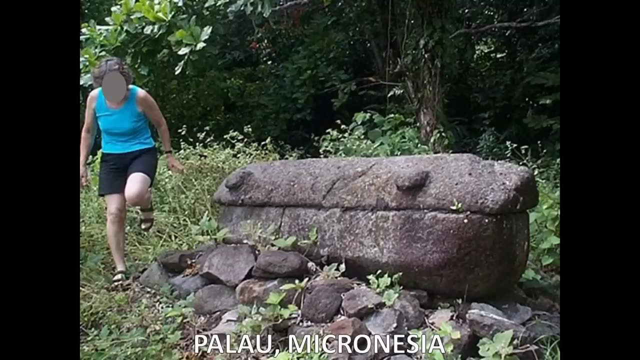 But even if we head to the remote Micronesian island of Palau, where there is at least one example of nubs on another sarcophagus, I'd be curious if there were other examples that existed on the island, which I bet if there's one, there's more, Even as we head west to the islands. 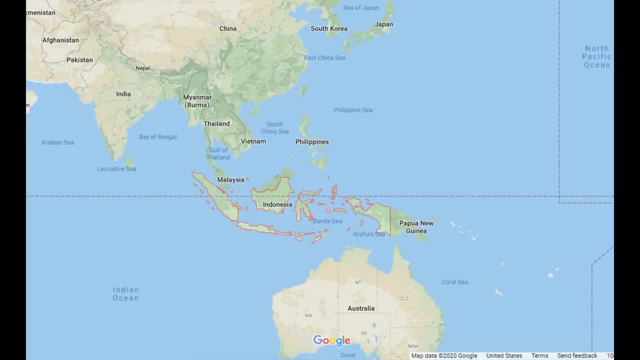 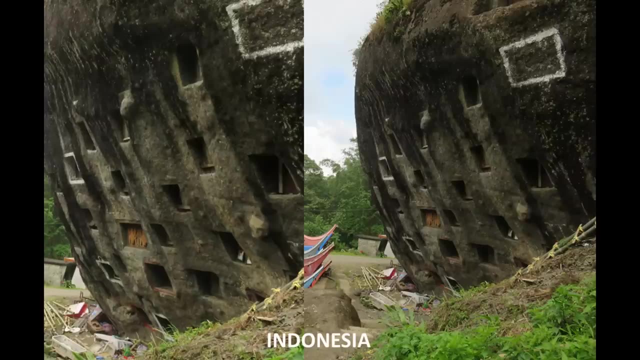 of Indonesia, where I already shared the fascinating similarity between the Moai statues of Easter Island, Peru and Turkey. well, you will also see examples of nubs here as well, and if you look closely, you will see more than just the few that grab your eye when you first see the image. 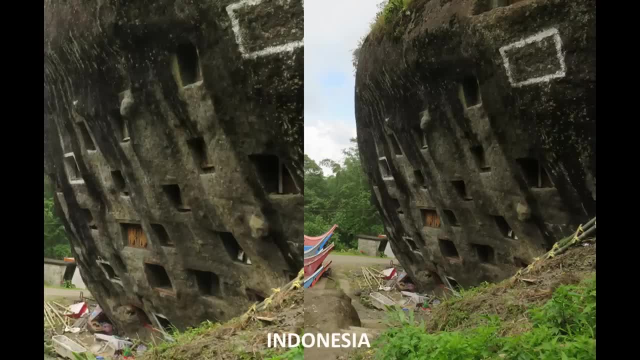 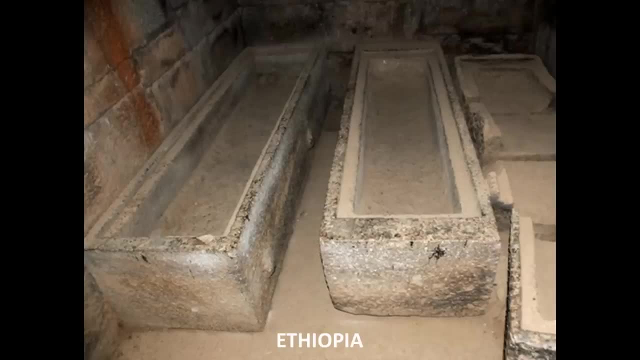 But I really wasn't kidding when I said that these nubs are all over. Even if we head back to Africa, to the country of Ethiopia, you can see nubs on a stone sarcophagus there as well, And if we head to the neighboring country of Sudan, to where most people don't even realize also has pyramids. 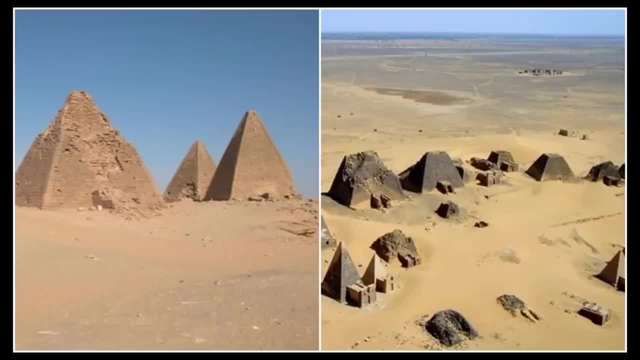 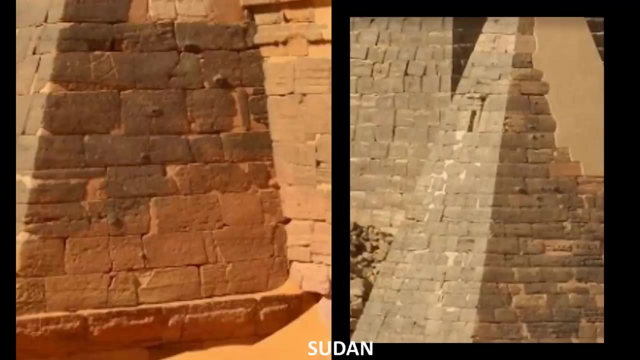 and of incredible precision, although much smaller than those of the pyramids of Giza. But someone please tell me if there are any other examples of nubs on the island and if there are any other examples of pyramids of Giza. And if you look closely, you will see nubs on some of the stones. 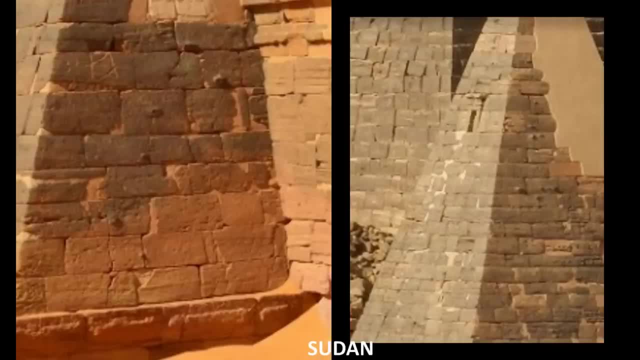 and keep in mind that these stone blocks are much larger than you realize, and so are the nubs, So these are not just blemishes. Hopefully we can get our hands on better photos of these pyramids and other nubs that may be found on them, But even if we head to Europe, 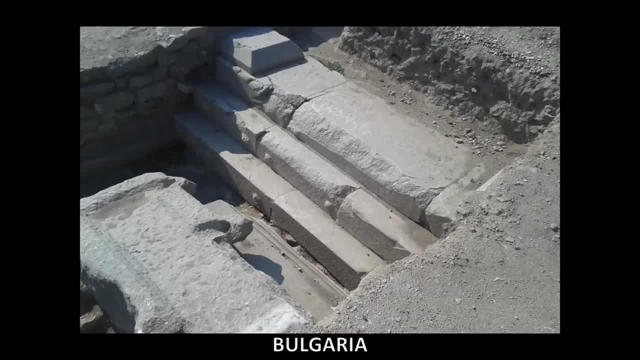 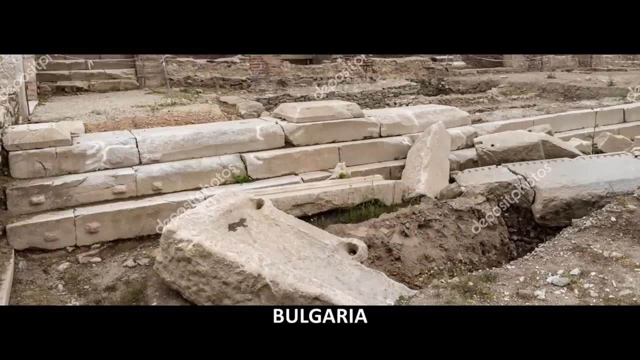 you will find examples of nubs in various countries, including Bulgaria, And again notice that the nubs are on some, but not all, of the stone blocks as well, like I mentioned at other locations. But we can even find examples of nubs in Syria, Again on some blocks, but most 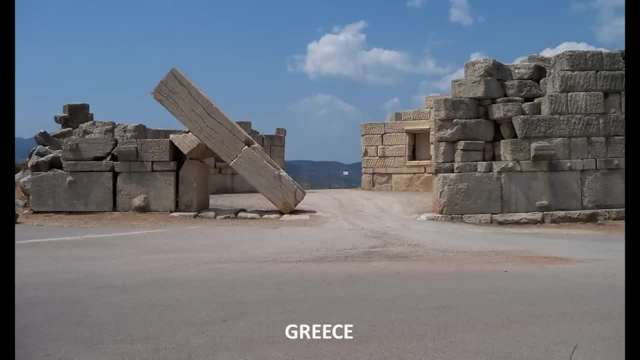 are without them, And if we head to Greece, there are a couple locations that have them as well. Interesting, though, that we don't find these nubs in Athens, at least from what I saw, And if they are, they certainly are not in abundance on the most popular ancient sites we know about. 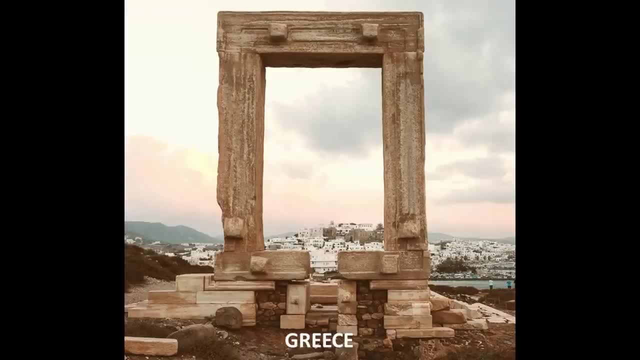 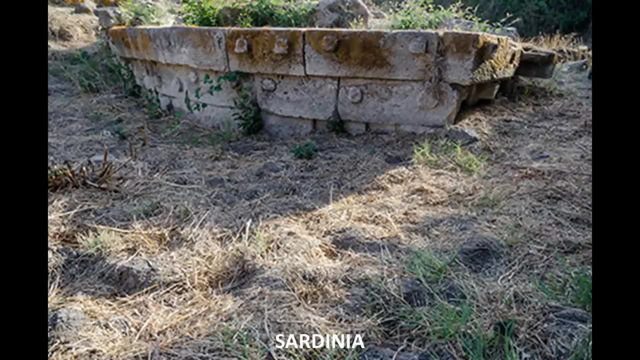 Even if we head to the Italian island of Sardinia, which is in the middle of the Mediterranean Sea, there are examples of nubs there as well. Same thing if we head to Turkey, where you can find an abundance of nub examples at various sites throughout the country. but for brevity of this, 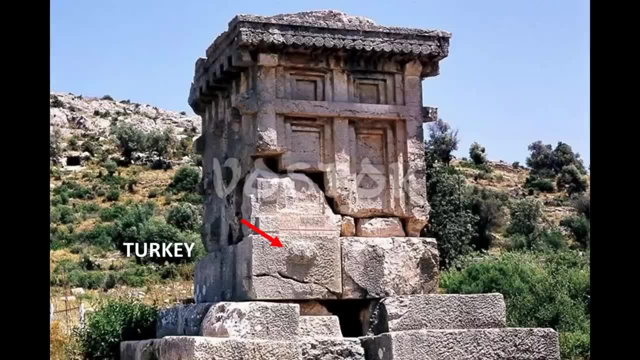 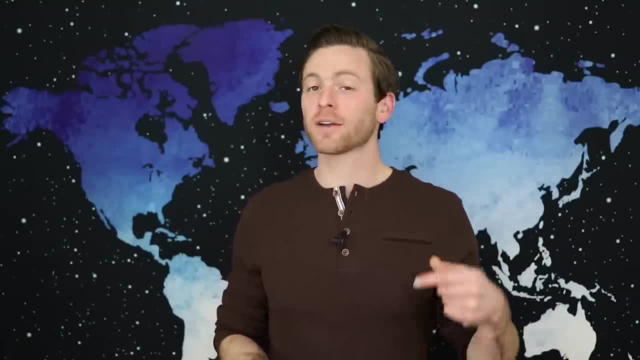 video. I'll show just a few to display the connection. But let me interject real quick here, since I just mentioned that there are nubs found in Italy and in Greece and elsewhere around the Mediterranean, and that there are nubs found in Greece and elsewhere around the Mediterranean. 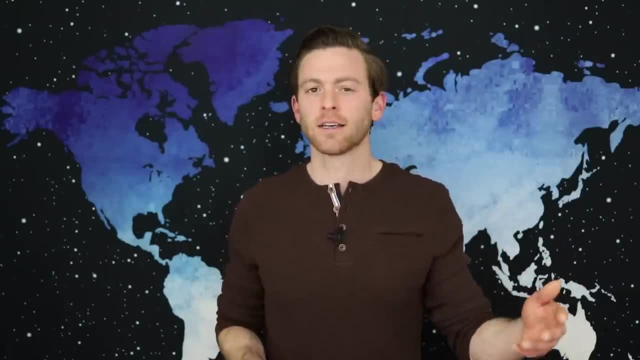 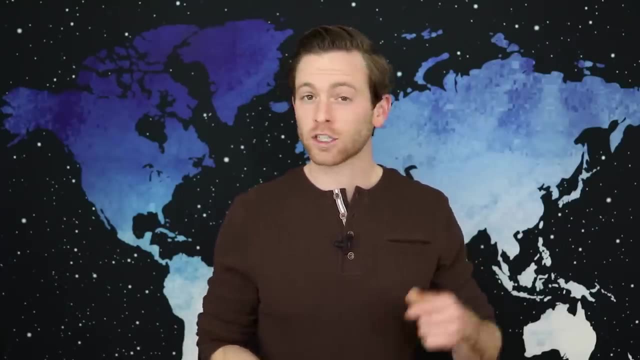 because some people might jump to the conclusion that hey, wait a second, this is just a matter of the Greeks or the Romans. but that can't be the case because, as we know, there are nubs in Japan, there are nubs in Peru, there's nubs in Indonesia and elsewhere. So if that were the case, that it 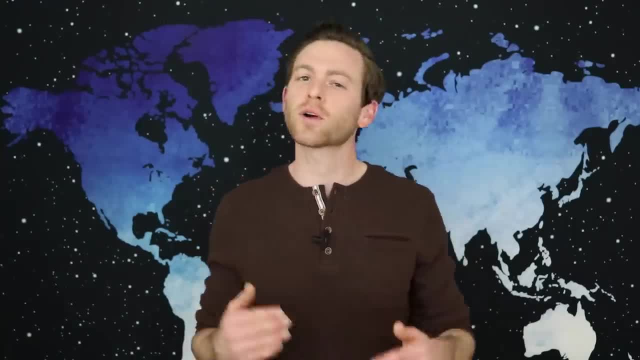 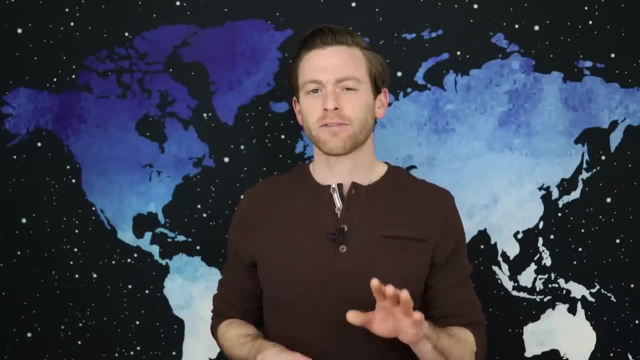 was just simply, oh, a Roman or a Greek thing, then why do we not see more examples of these one within their capitals, all over the place, within the notable tourist attractions that we always see and hear about, as well as the fact we'd have to say, hey, were the Romans or the 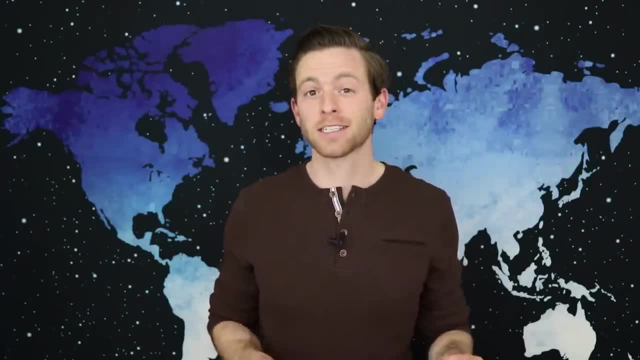 Greeks capable of traversing the Mediterranean Sea, or were they capable of traversing the ocean at vast distances? Because that would completely contradict what we learned in school as well, and what the scientific community say is even possible. So something to think about. 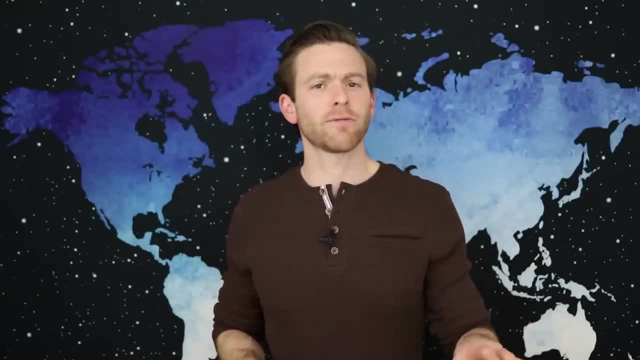 So, with that said, it seems to me that, at a minimum, based on what we've seen so far, the widespread nature of these ancient nub phenomena and these other aspects we've shared so far in the video- that at a minimum it shows that, regardless the ages of these things or who, 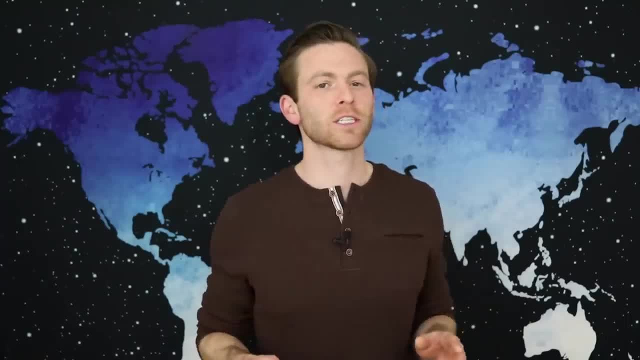 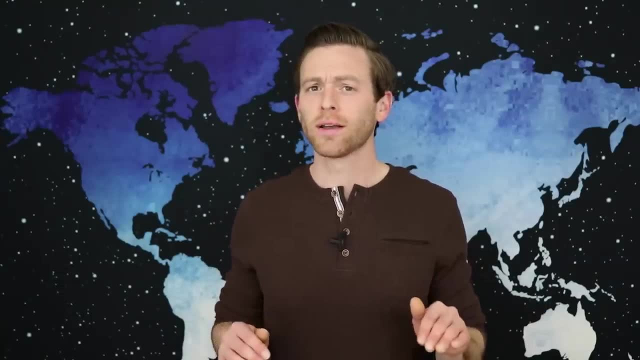 made them that, at a minimum, there's far more to the story of what we thought we knew about our ancient past as it is, And that's what we're going to talk about in this video. So let's get started. Regardless of the age or who did it, there's clearly something more that we don't know about. 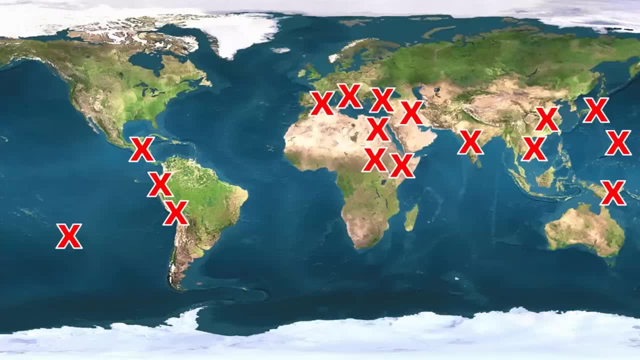 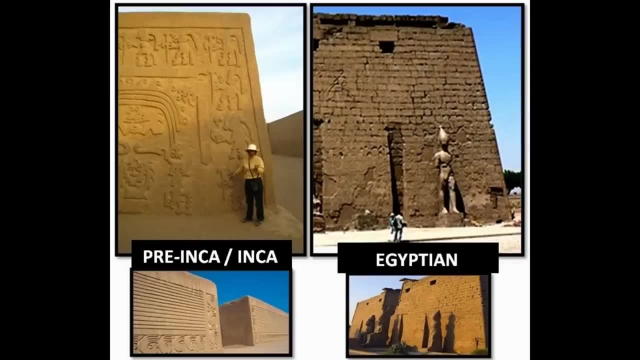 Now let me keep going because I have more to share. So in previous videos I've shared unique comparisons between angled structures of ancient sites in Peru to that of Egypt, and these are just a couple examples. Now I've also shared examples of that of trapezoidal doorways. So let's head. 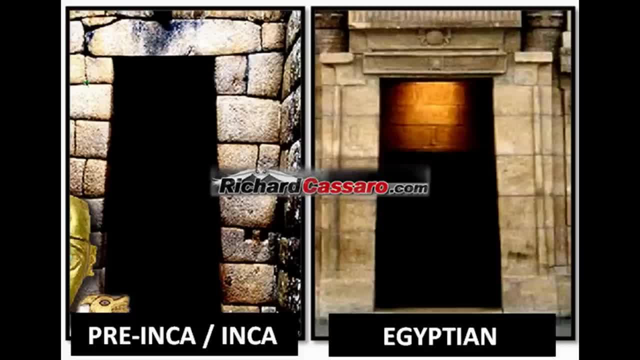 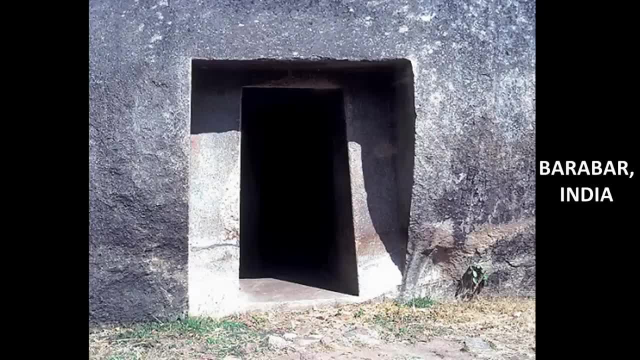 back to ancient sites within India. Look at this here. cut out of solid stone, Make no mistake. these symmetrical angles would have made the construction far more difficult to do compared to a straight line, And I'll give further supporting evidence of that in a second. 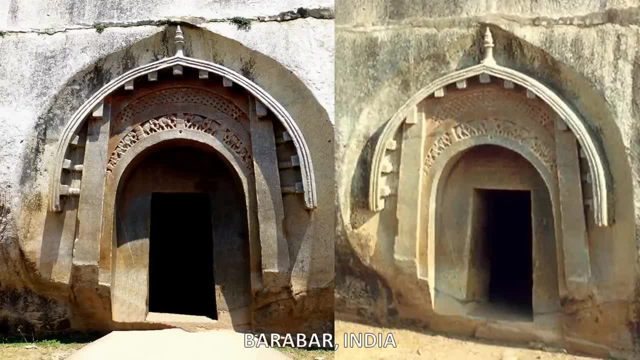 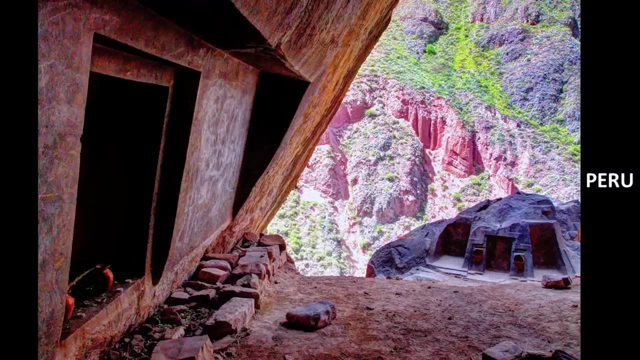 but look at these various different trapezoidal doorways first. Now let's head to the opposite side of the world again, to South America. Let's first notice the cutout itself, which is not exactly the same as in India, but similar, and with great precision. 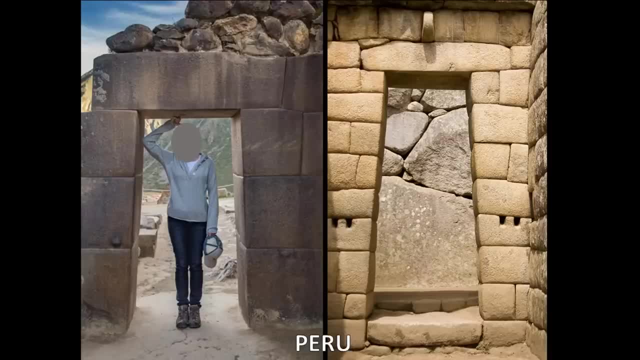 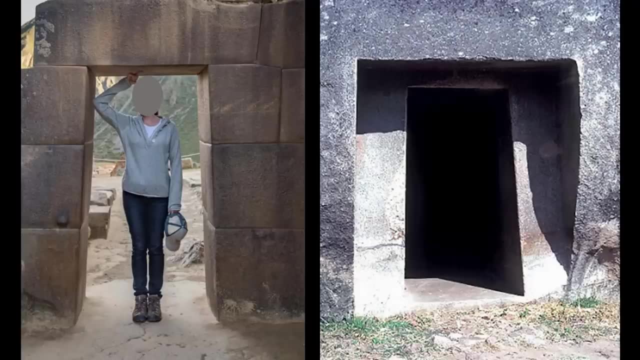 and equally difficult to accomplish. Now look at just a couple examples of trapezoidal doorways in various places throughout Peru. Of course, not exactly the same as within India, as these sites in Peru utilize separate stones rather than just one solid stone cutout. 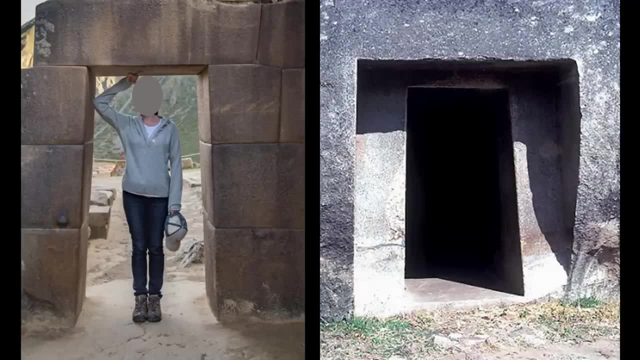 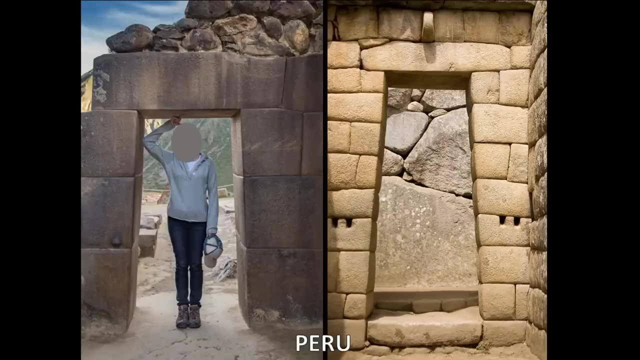 But to emphasize my point that the trapezoidal design is far more difficult than straight lines, you have to appreciate that it would be far easier to cut a bunch of square or rectangular stone blocks of the same exact dimensions and then stack them upon each other. 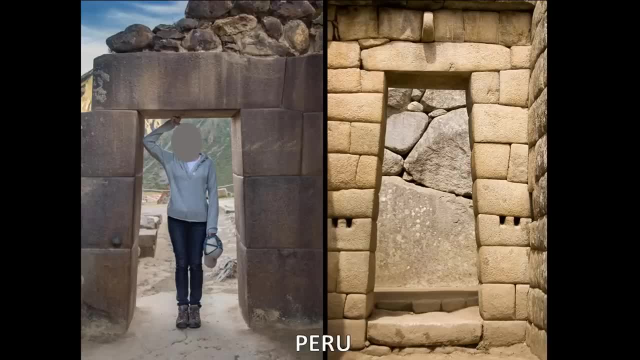 into the design of a doorway. But when going the route of a trapezoidal design, each layer of block is a different shape than that of the one above or below it in order to achieve the symmetrical angle That right, there is next level difficulty. 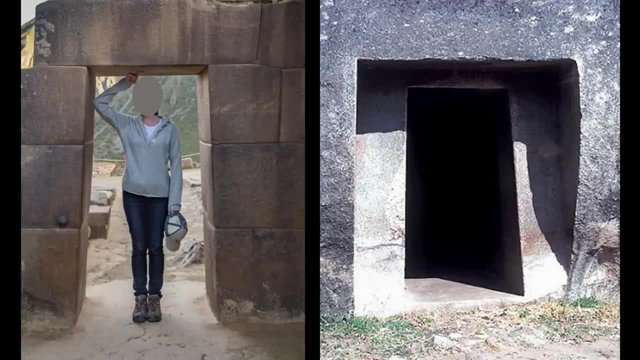 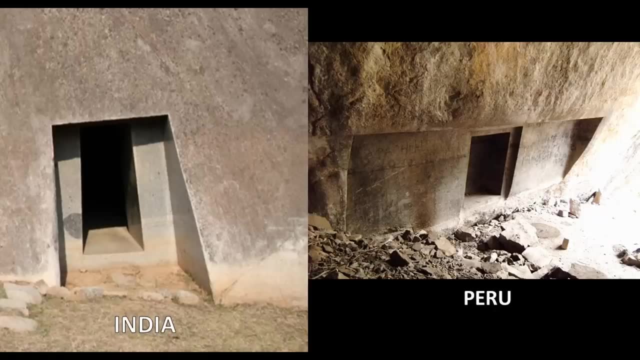 Now again, this is not exactly the same as in India, but let me remind you again of the example involving the skyscrapers across the world: All different types of architecture. none are the same, but they're still essentially the same thing, just different. It's worth mentioning that these are 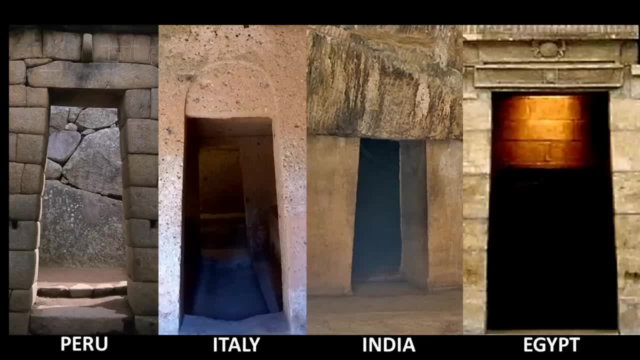 only examples of trapezoidal doors you'll find around the world, though. In fact, a certain place in Italy has trapezoid doors, and this feature can even be found in ancient Egypt as well. Isn't that interesting And real quick. the site here in Italy is in Lazio, and it was a tomb. 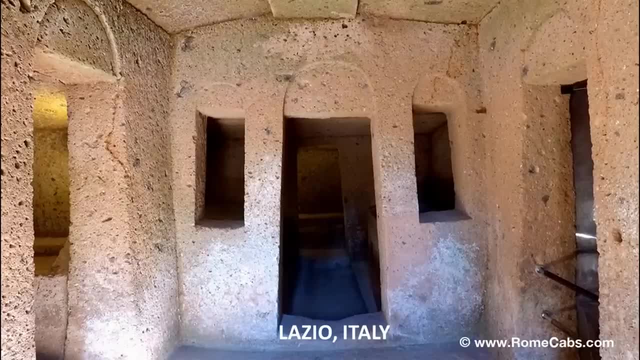 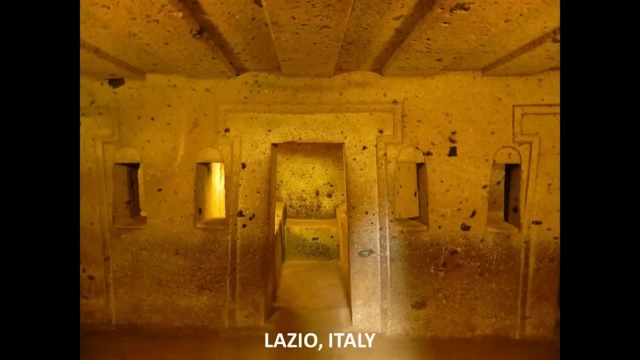 Take a look at a few different photos here, Observe not just the shape of the doorway but also the windows, And notice that it has false windows as well. Now let's compare that to Peru and tell me what you think about it. Let me know in the comments below If you liked this video. 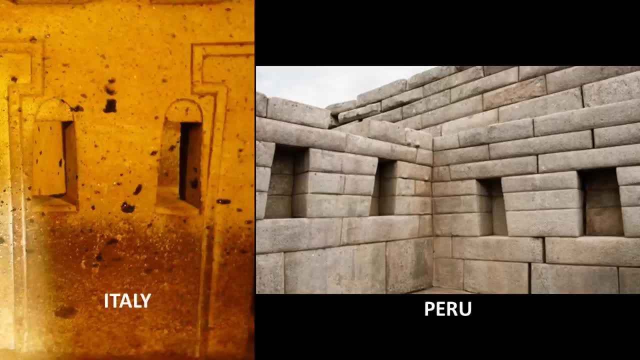 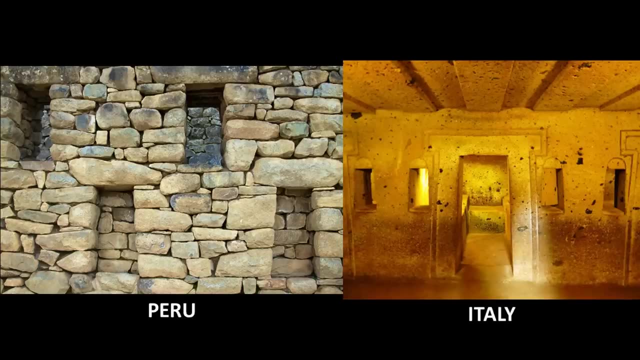 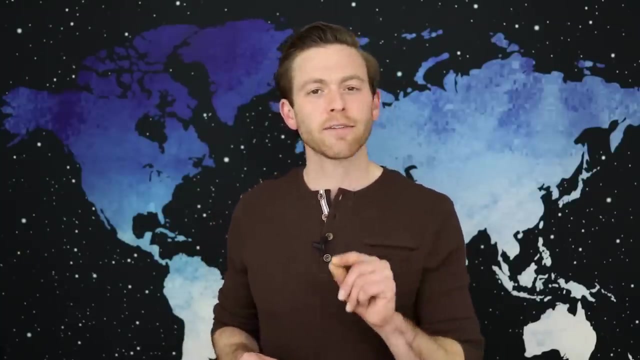 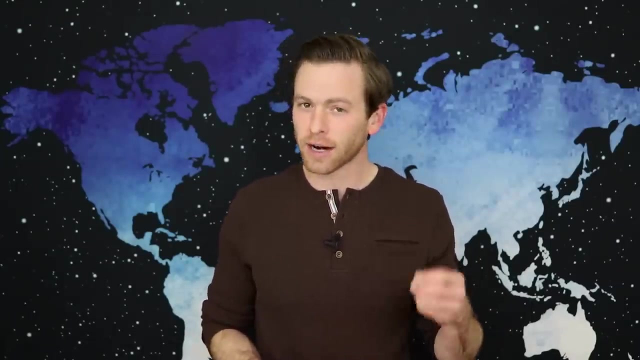 leave a like and subscribe to my channel for more videos like this. Thanks for watching Now. I had a career as a corporate fraud investigator, where I would investigate employees that were suspected of stealing and defrauding the company, And I would gather evidence and build. 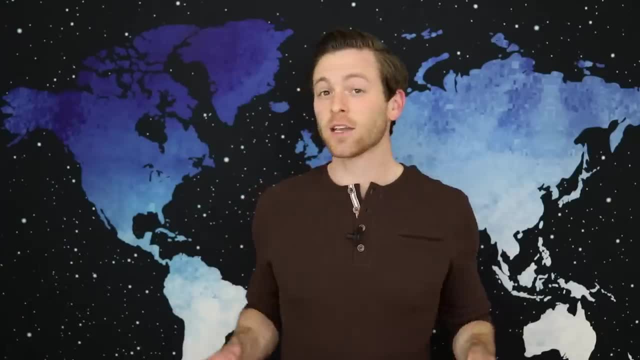 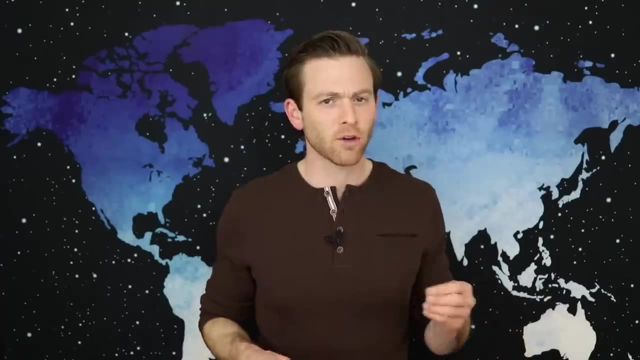 a case that would eventually lead to an arrest and prosecution. And what I can tell you is that, in the court of law, regardless of the crime that if you don't have you know caught red-handed on video tape or something of the crime- what you do is you build up a bunch of points of evidence. 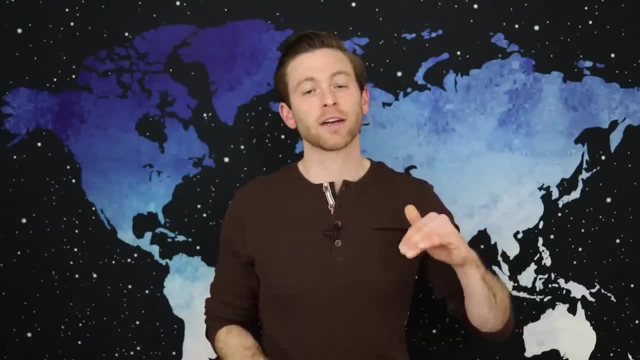 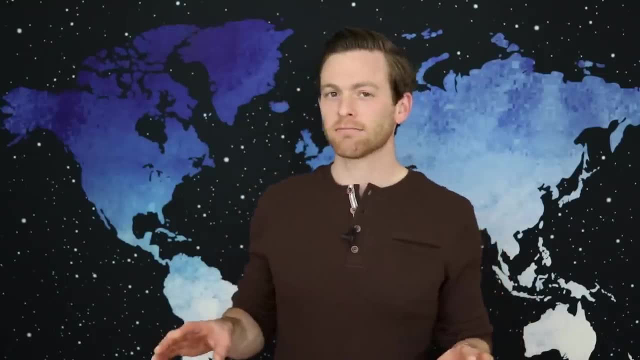 line items of evidence at this place at this time, and you gather and you gather and eventually all those lines of evidence lead to what's considered proof and will lead to a conviction. So let me ask you this: When you look at all the information that I've shared in this video, all the physical evidence, the details, 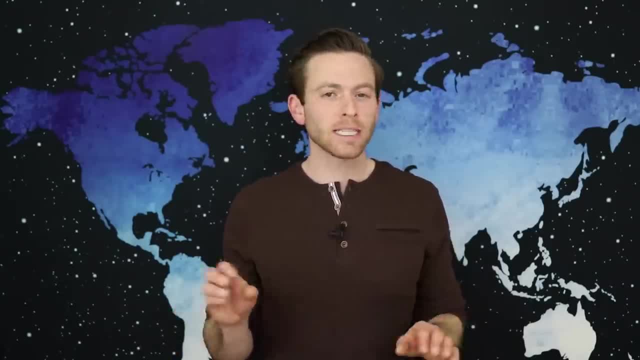 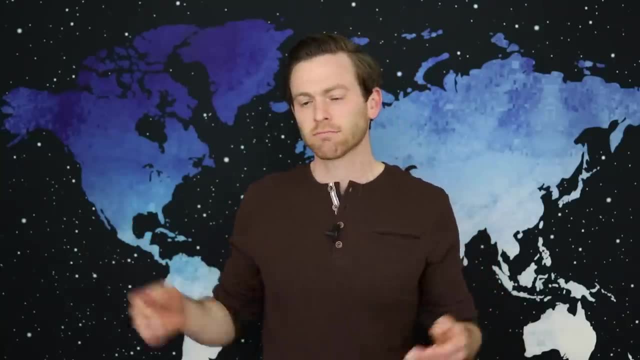 is it really just a coincidence? Or when you piece it all together and you look at all the information together as opposed to individually, because you could write anything off. Oh, trapezoidal door, it's possible, that's just a coincidence. The tridents coincidence, All of. 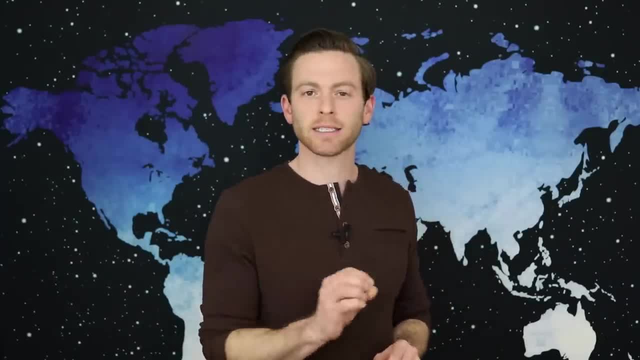 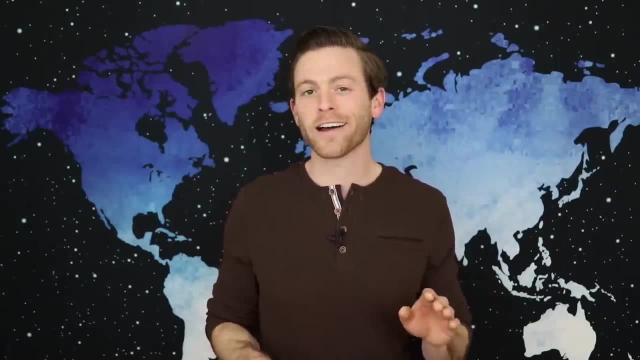 this could be just a coincidence and inconsequential when you look at it by itself, But when you bring it all together, does this not amount to actual proof that clearly there's far more going on in this case than there is in the court of law, If you look at all the information? 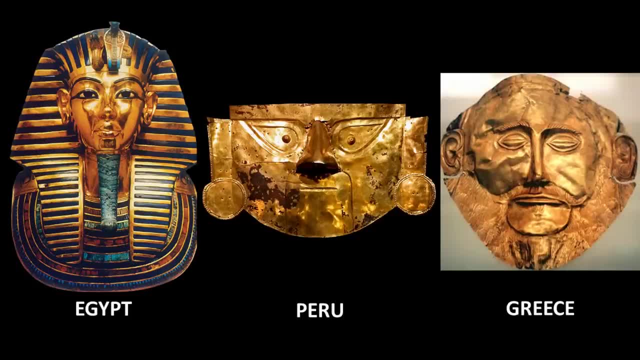 you have gathered. what does that mean? What even is going on in our ancient past and what we ever thought I mean? let's review real quick. We have gold funerary masks among three separate and far apart cultures that are supposed to have no connection to each other at all. 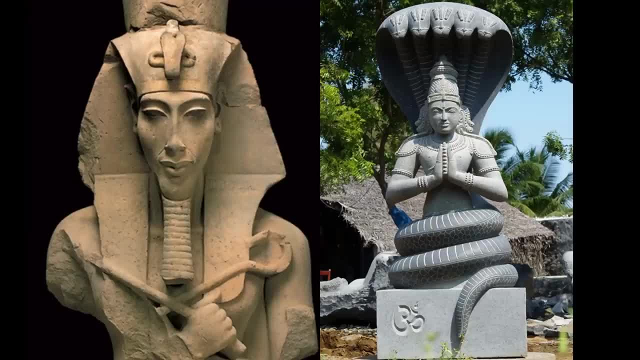 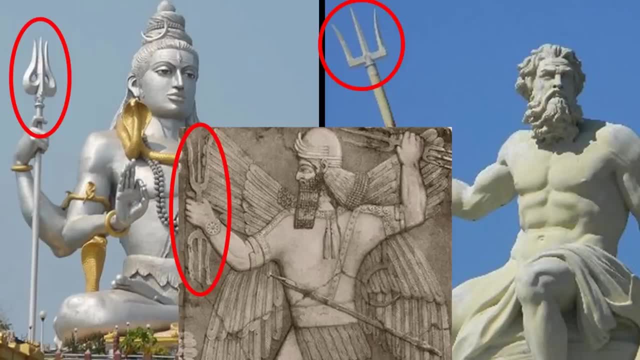 We have depictions of cobra snakes at the head of two different cultures, along with depictions of the caduceus among three different cultures, along with depictions of the tridents among those cultures, depictions of handbags etched in stone, separated by, in some cases, tens of thousands of. 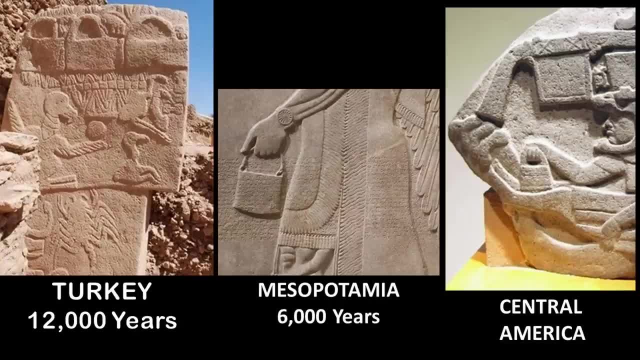 hands of stones separated by, in some cases tens of thousands of hands of stones separated by in thousands of years, when you consider Gobekli Tepe to the connection of the Olmecs in Mesoamerica. I mean, really, is that detail just a coincidence? How? 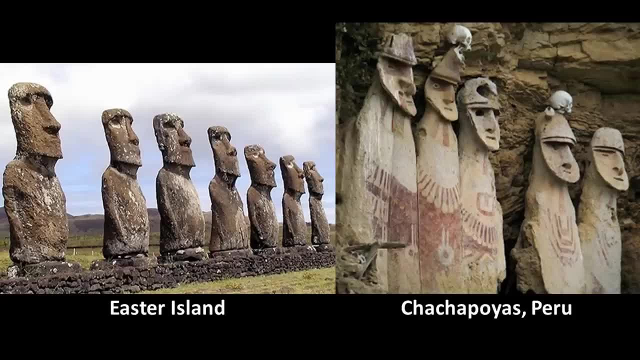 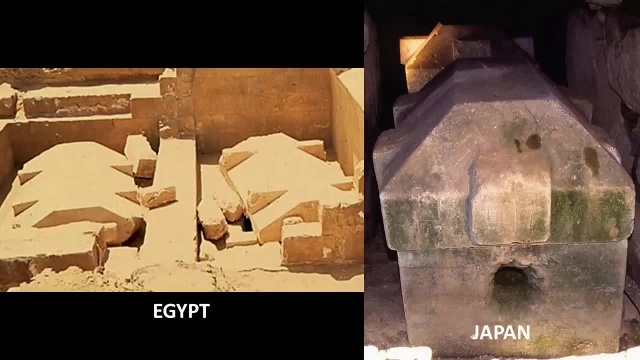 specific can we get? We also have the creepy similarity of the Moai statues to others in Peru, Turkey and Indonesia. We also have a bizarre similarity between Egypt and Japan, when you consider that stone box sarcophagus and how similar they both look and having had no connections between those two cultures, 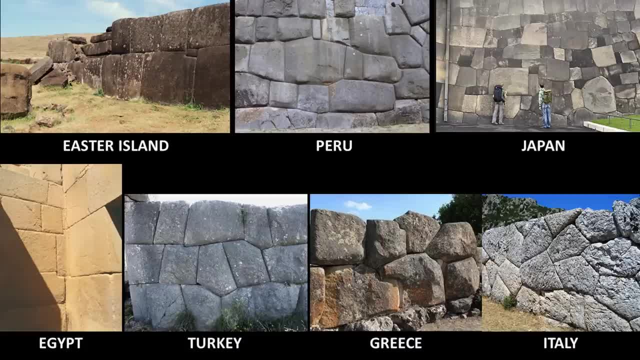 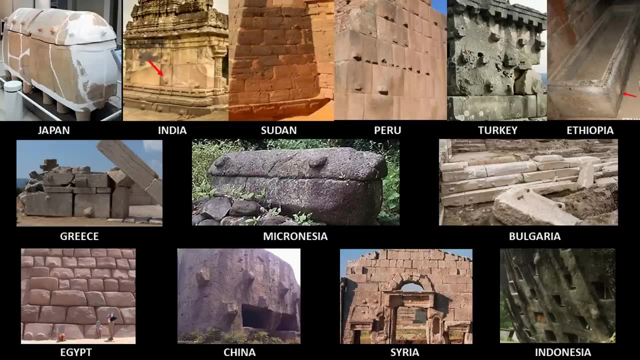 that were a world apart. We also have polygonal stone blocks found throughout the world, ranging from Easter Island, Peru, Egypt, Japan and throughout the Mediterranean, And we also have the stone nub phenomena that are found across the world, including, again, Japan, Micronesia, Indonesia, Egypt, Peru and again. 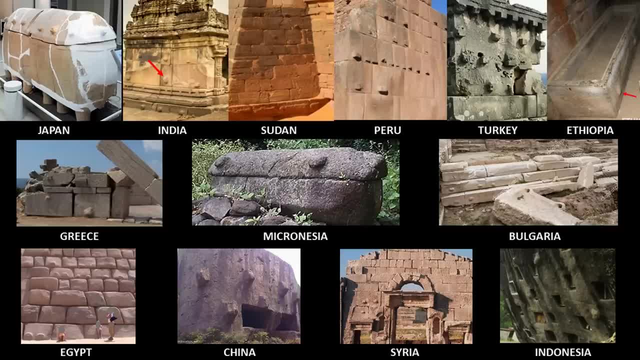 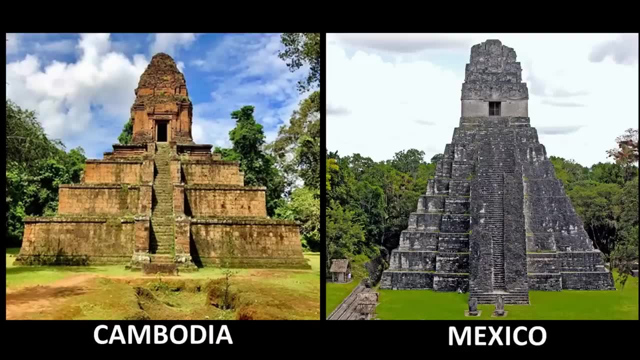 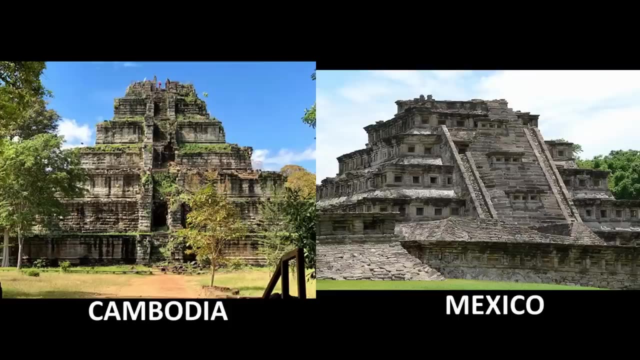 throughout Africa and Europe. Consider all of that and now take a second look at the similarities between the pyramids of Egypt and the stone blocks that are found across the world. Do these side-by-side comparisons really suggest a simple and natural evolution of structural design that are totally organic and natural within itself, Or is 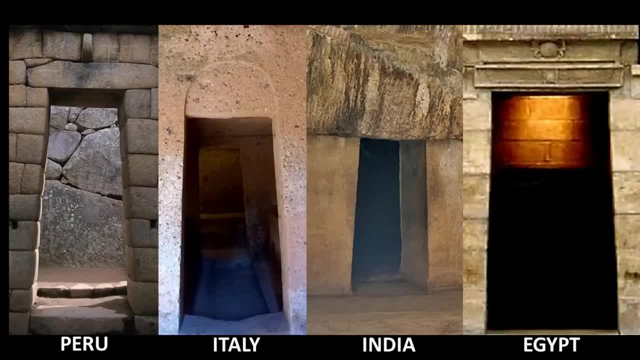 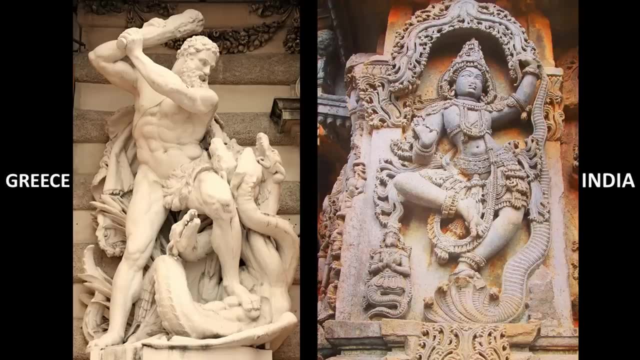 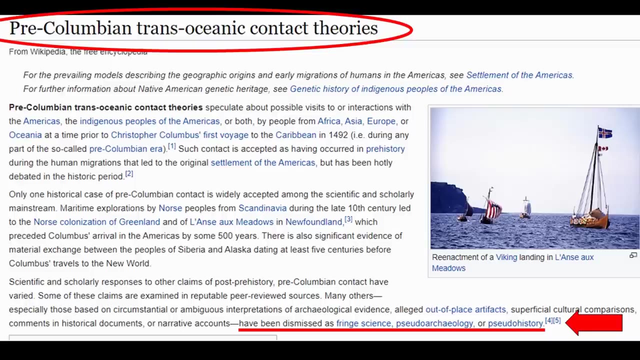 it. when you study the specific and truly unique aspects and in combination with everything else shared in this video, does it seem to be more than just a coincidence? Academics profusely reject an ancient global connection or civilization of any kind, and they ridicule the other's that suggest it with essentially name-calling. you know words. 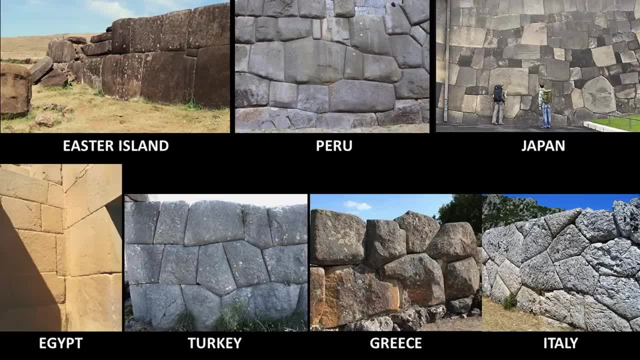 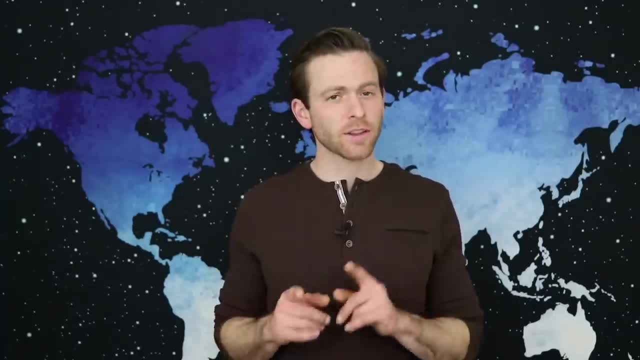 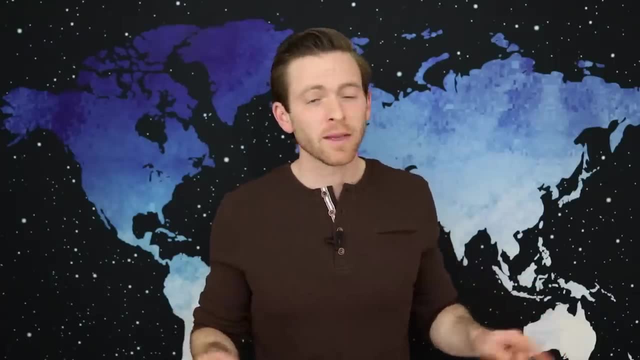 like fringe and pseudo, Yet they never actually go through and share all of the details with those who they intend to persuade. Look at all these details that I've shared in this video and think for yourself. And isn't it interesting that none of these things were shared with you in school at all, In fact, only a very 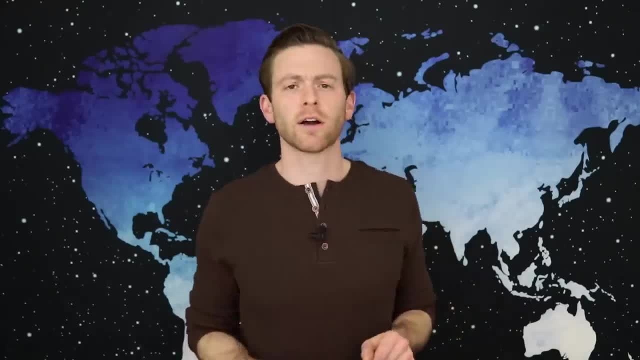 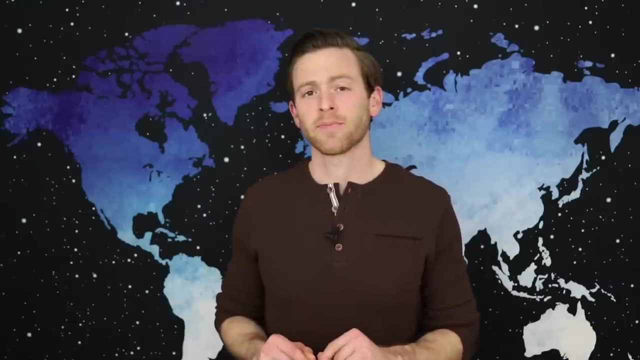 small percentage of people have seen some of these details before. Of course there are ancient history enthusiasts that watch this channel, that are subscribed. there are other youtubers. I'm not the first to talk about these things, although I can tell you that while researching this topic in the last 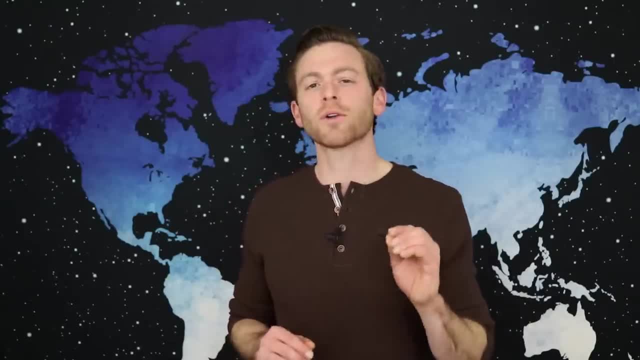 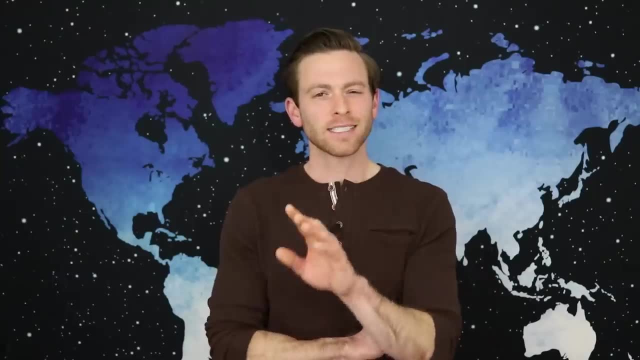 number of weeks that many of these things. I was blown away. my jaw dropped at seeing the connections between Japan and Easter Island and elsewhere around the world that this, this adds up far more than I thought. I was already suspicious and thought that there was a global civilization. I think a lot of. 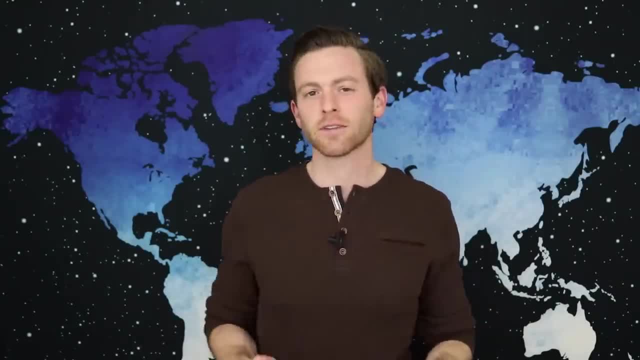 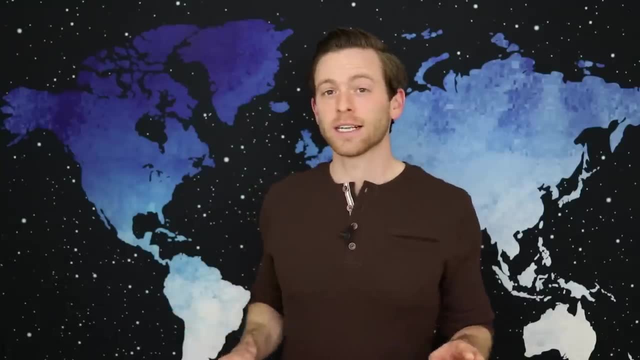 people that watch this channel and are enthusiasts for the topic of lost ancient civilizations. they already knew it, But where do you Were they aware of the extent of all of this? I don't think it's a coincidence, but that's not to say that we should just start rewriting. 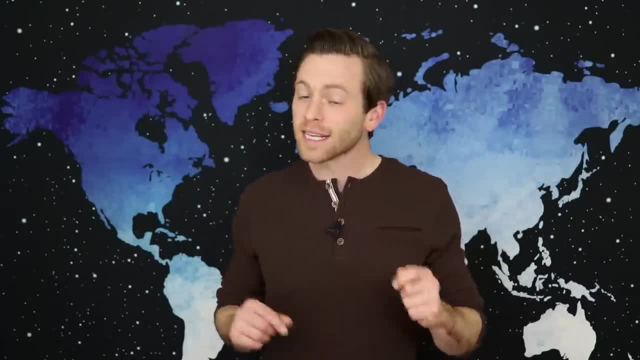 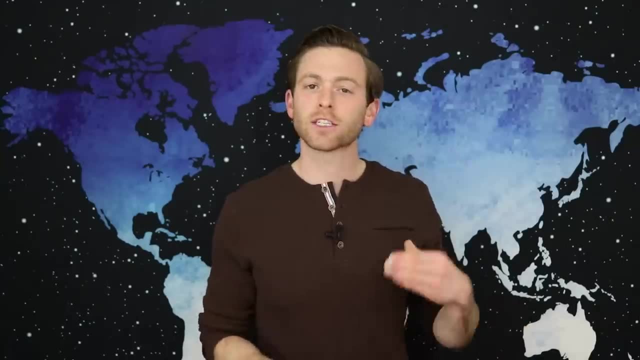 the textbooks. right. this second, But at a minimum. what is necessary is a whole new conversation and debate, And these details should at least be presented to the younger generation that is currently in school now, Because, keep in mind, this stuff is shunned right. 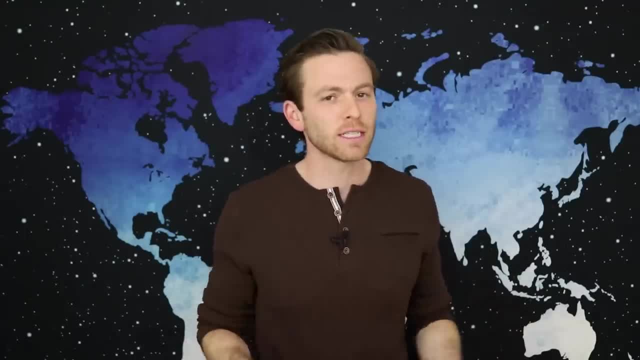 Even people that study this stuff are oblivious to a lot of these same little details, right? So, with that being said, there's going to be a whole new generation of academic scholars and archaeologists and historians that it would be great for them to be raised with. 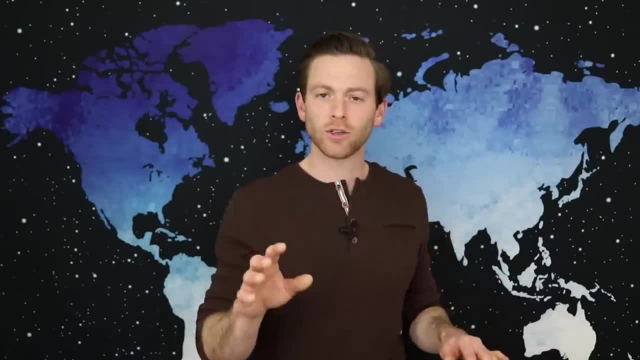 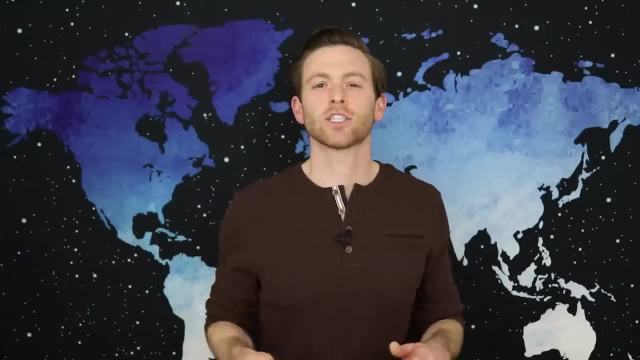 a more open mind, Because what happens is people are raised into being told one thing, and then they grow up thinking the same thing, And then, when they hear something new as an adult, they're like: wait, that's not true.